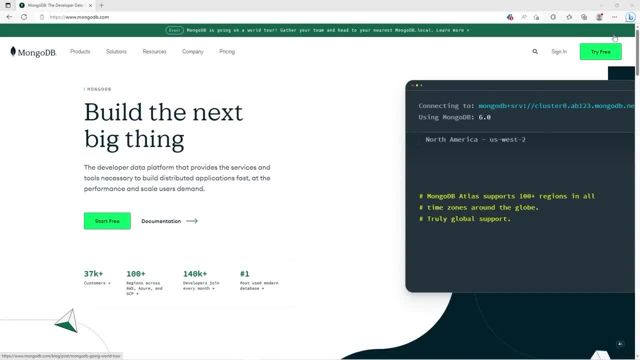 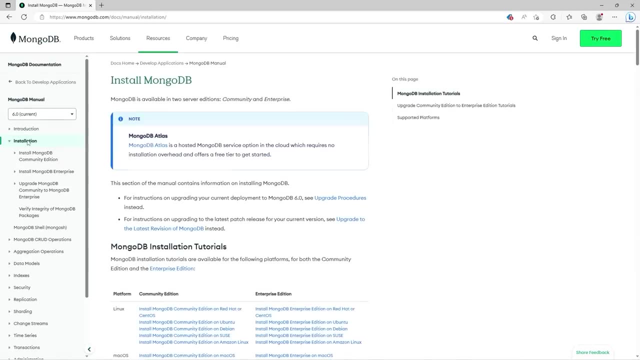 you what you need to download. All right, let's get started, everybody. Here is the installation process for MongoDB. So go to this website, mongodbcom. Go to resources server On the left sidebar. go to installation. There is a list of different installation tutorials, depending on your operating system. 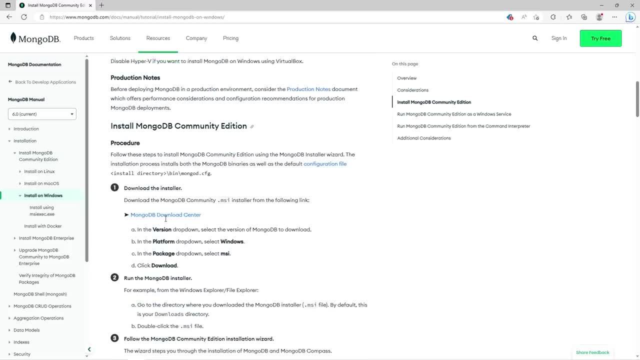 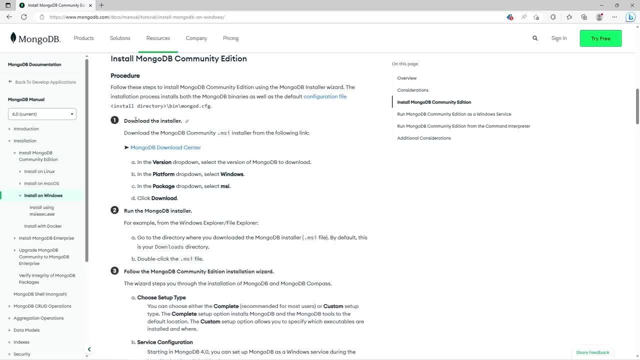 I'm running Windows. I'll select Windows. Let's scroll down. We are looking for. install MongoDB Community Edition. All you have to do is follow the numbered steps, Beginning with one. we will go to the download center. I'll open this in a new tab because I don't. 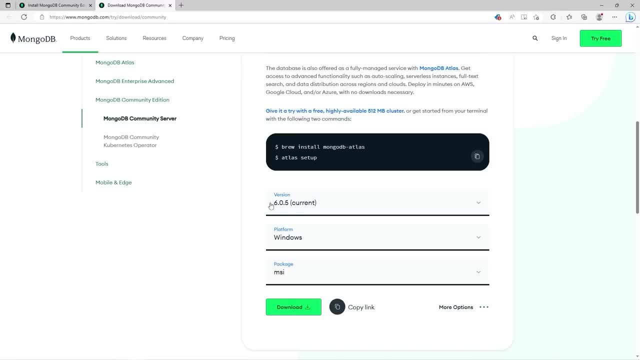 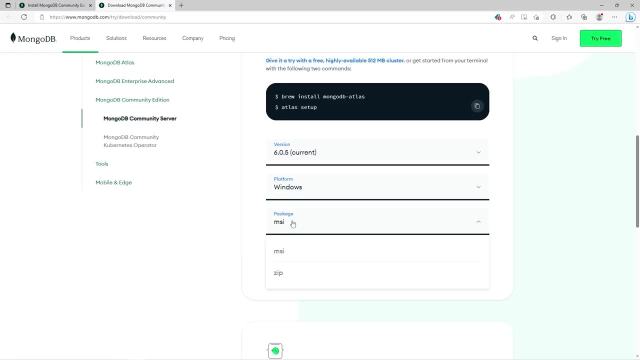 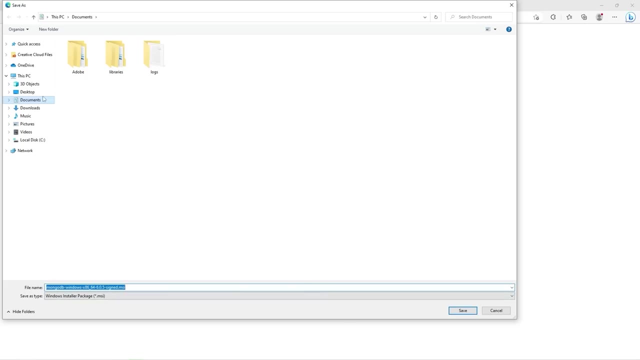 want to close out of this window. Select the current version. Select your platform. Again, I'm running Windows. I'll keep that the same And download. Pick a place to save the installer to. I'll keep it within my documents folder, but you choose your own place And I will open this when it's done. 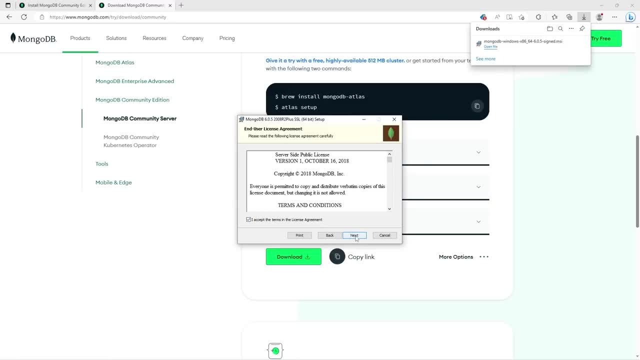 So we're going to click next: Accept the license agreement. Next, Complete: Install MongoD as a service. Make sure that's checked. Next, Also, be sure to install the MongoDB Compass program. It's a graphical user interface. Then give it a couple minutes, Now that MongoDB is installed. 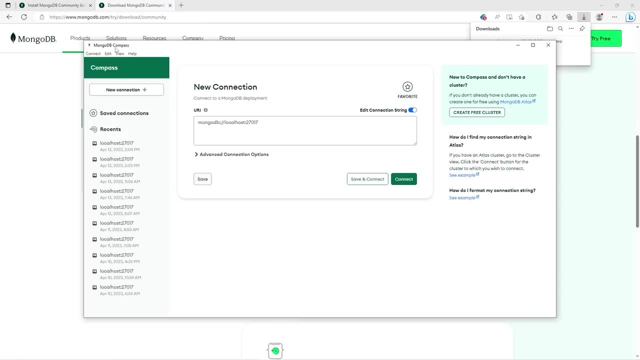 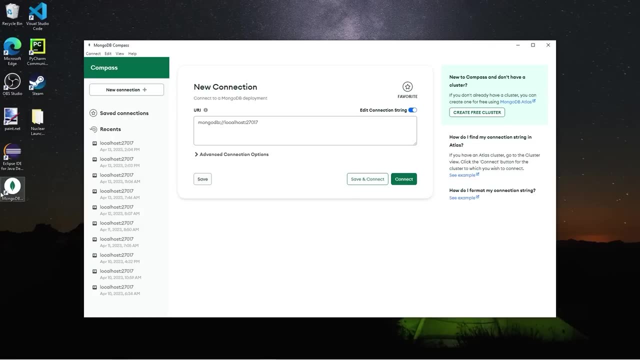 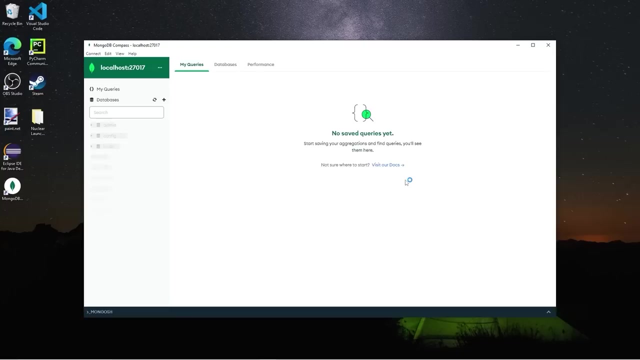 we can finish. This may open Compass. Compass is a graphical user interface for managing our database. We'll be using Compass intermittently. In fact, I recommend creating a desktop shortcut. You just have to open it. Then, to establish a connection, you hit the green connect button. 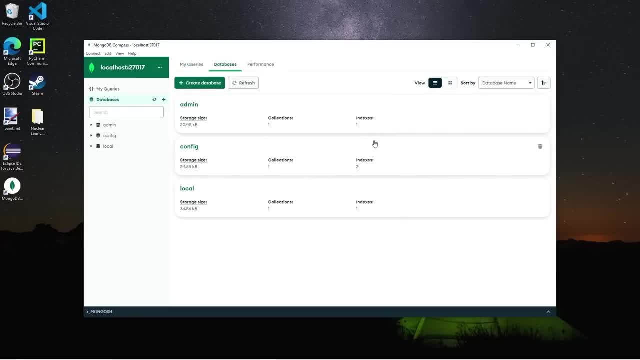 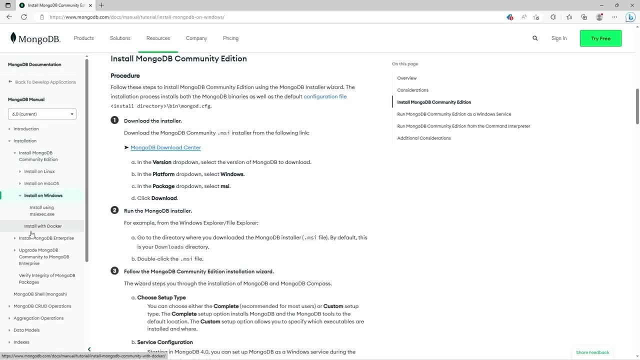 I'll be using Compass intermittently just to show you how everything works. Let's also install the MongoDB shell. To install the shell, we're going to go to the left sidebar And where is it There: MongoDB shell, Also known as Mongosh, Like. oh my gosh. 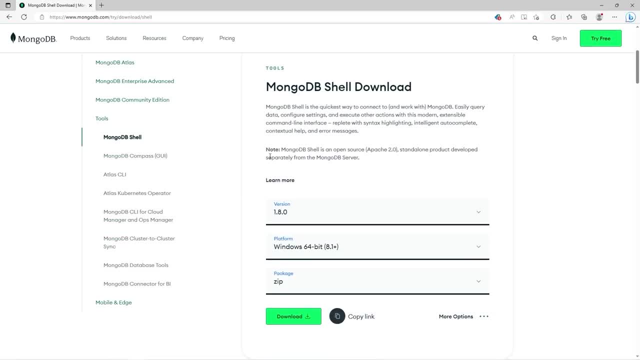 We are going to go to the download center. Select the current version. Select your platform. I'm running Windows And the package. We'll keep that the same And download. We'll open this. when it's done, We will unzip this And we're going to go to the download center. And we're going to go to the. 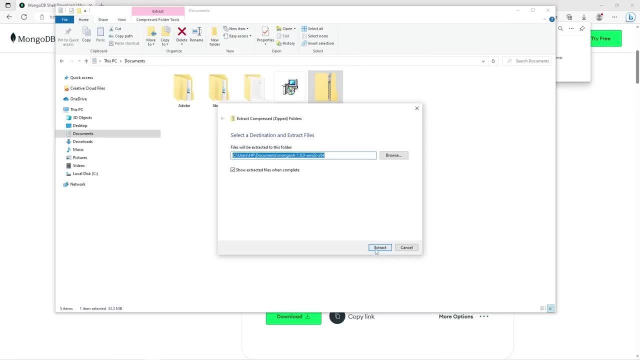 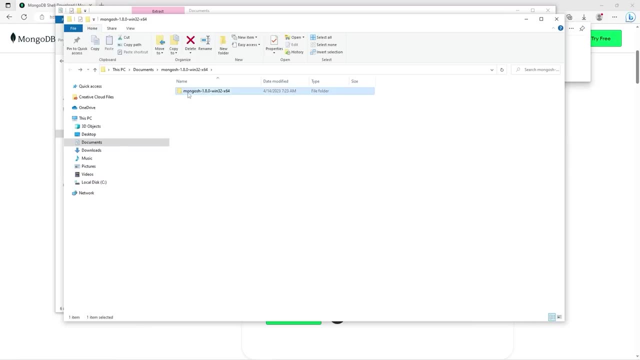 folder. So right click, Extract all. We will need the file path to the executable. Let's open this folder, Go to bin And we can copy this file location. Let's right click on our executable, Go to properties. Copy this file location. It should be within the bin folder. 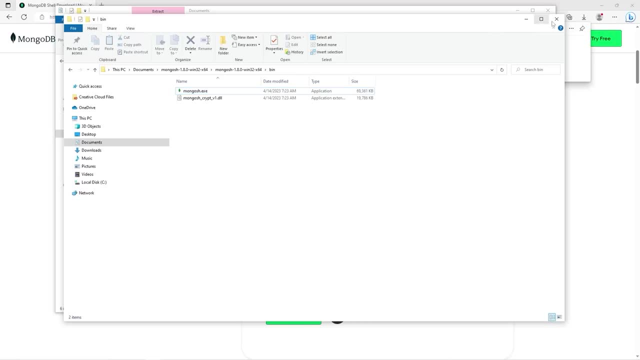 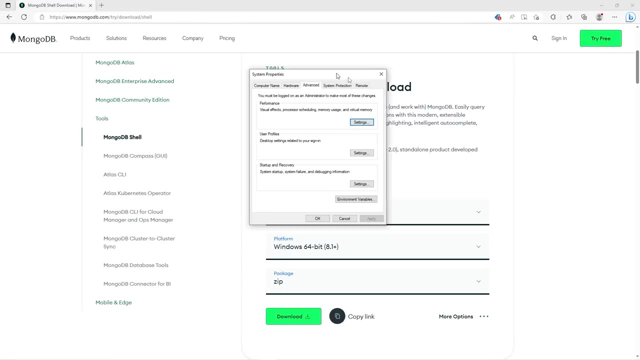 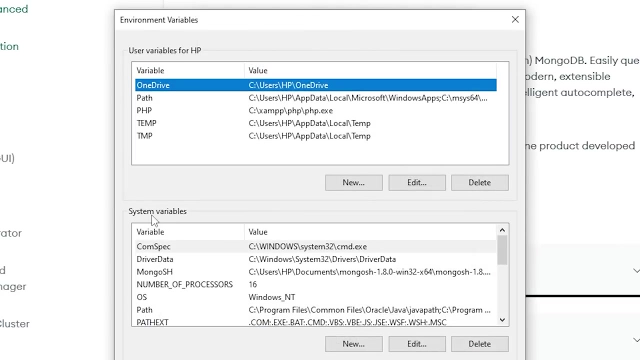 Then we're going to add that file path to our environment variables. Really, we can just search for environment variables. We're within system properties. Go to the advanced tab, Environment variables, Underneath system variables. Let's pretend that this wasn't here. Click new, Come up with a. 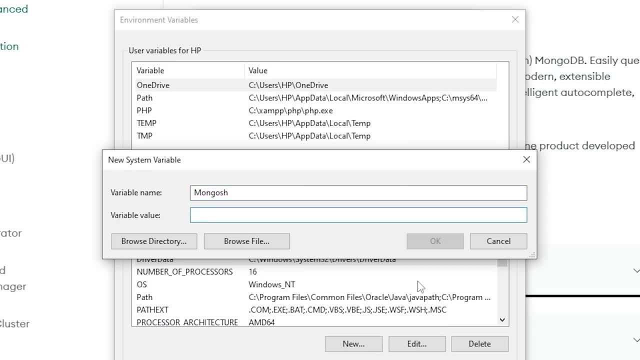 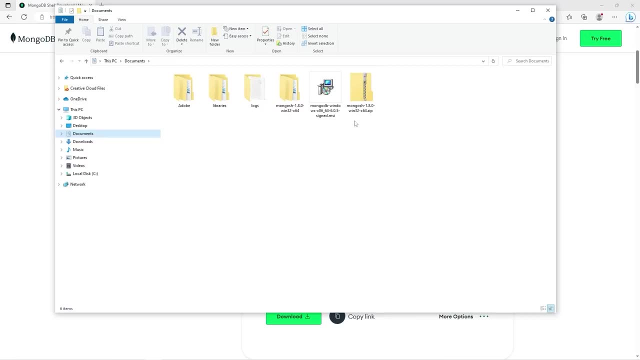 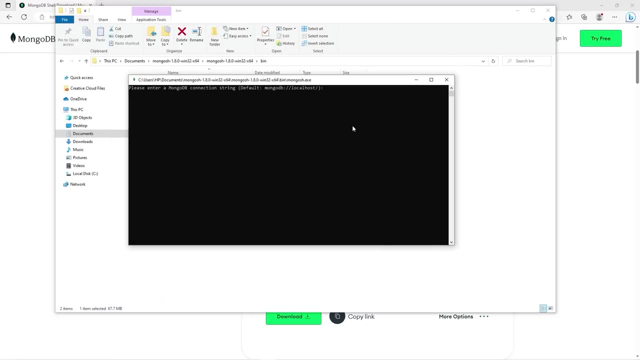 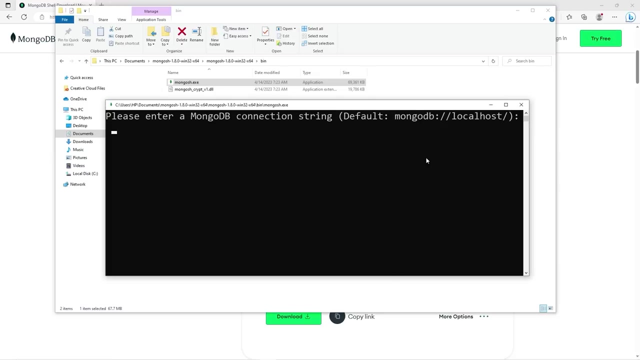 variable name Mongo SH is good, Then paste that file location, Hit okay, Okay And close. So if we want to open that folder And open the executable, This is the MongoDB shell. I'm going to make the font size a little bit bigger To establish a connection to our database type: Mongo SH. 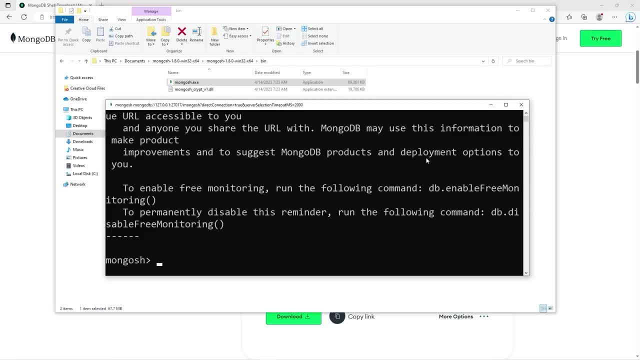 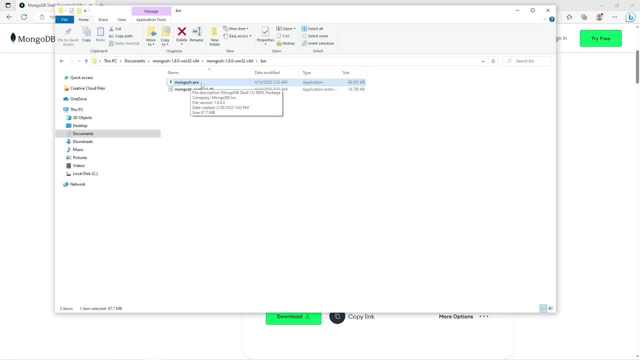 And that should establish a connection To clear your screen. type CLS To exit. type exit: Personally, I don't like using this executable by itself. I like using VS code. If you would like to use VS code for using the shell, here's how. 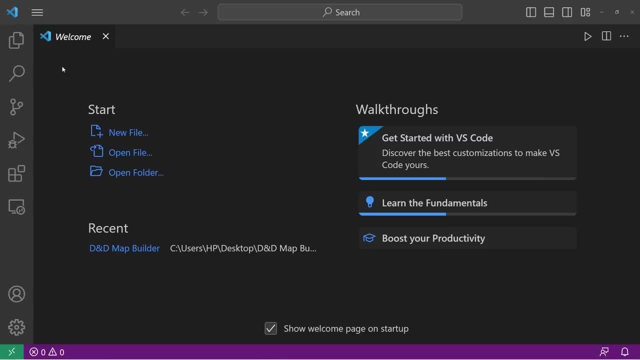 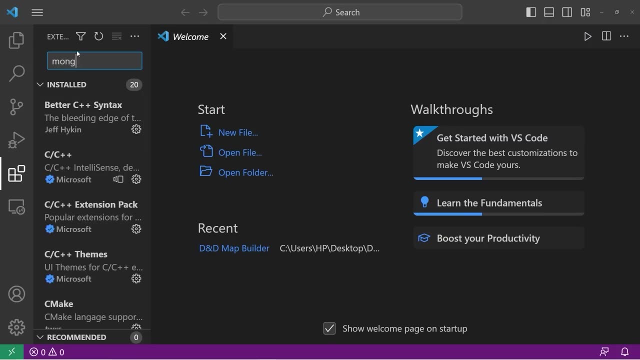 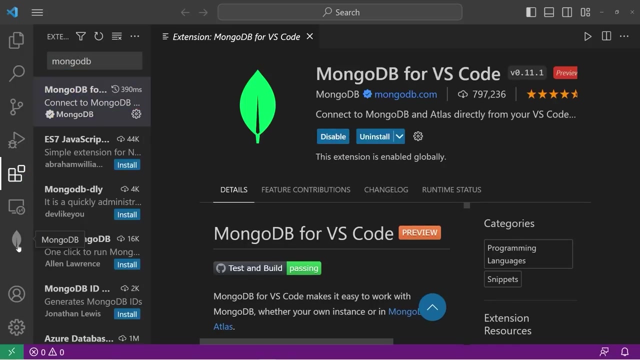 If you would like to use VS code for using the shell, here's how. So, within VS code, we're going to download the MongoDB extension. So go to extensions, Search for MongoDB. It should be this one. We will install this extension. There should be a new icon for. 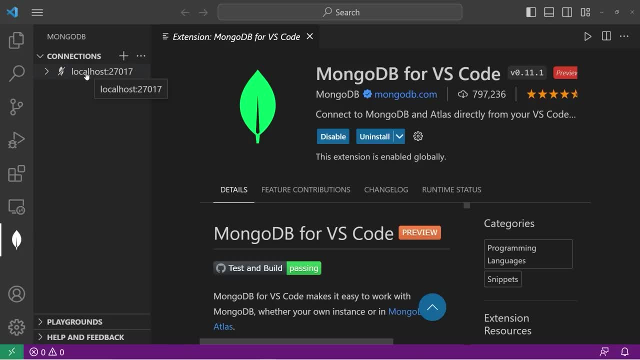 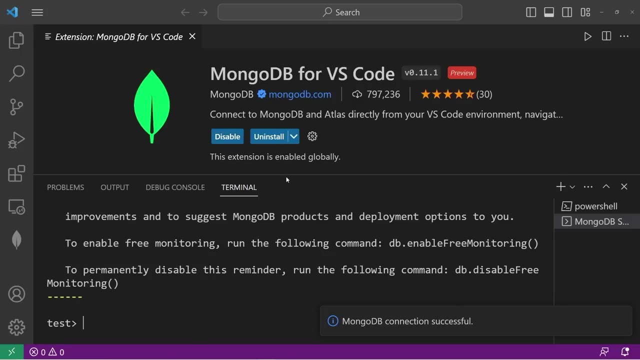 MongoDB. Let's click on it. To establish a connection. we just have to click on local host. The MongoDB connection was successful. Then, to open our terminal, right click- Launch MongoDB shell. Let's minimize this. Close out of this window. Pull up this terminal. 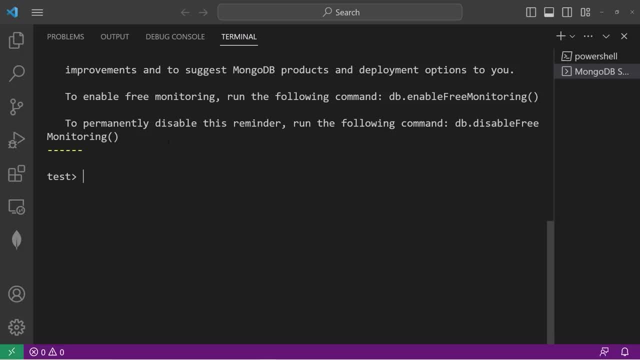 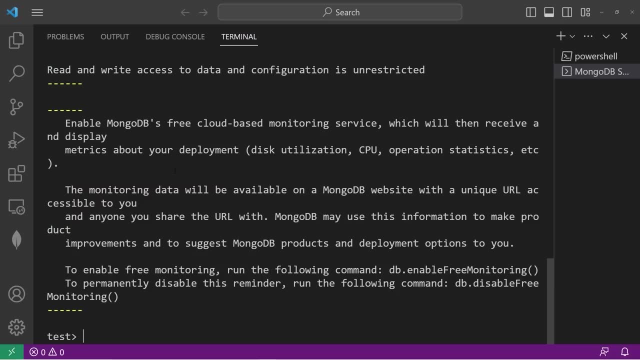 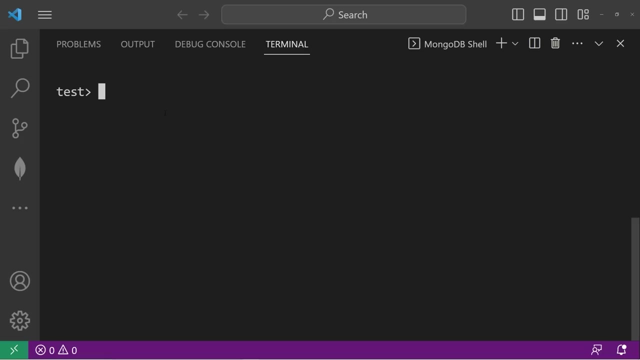 We are utilizing the MongoDB shell with VS code. So to exit, you type exit. To establish a connection, you can type Mongo SH. To clear your screen, you can type CLS, And that is everything you need to know to get started. Hey everybody, Here's how we can create and. 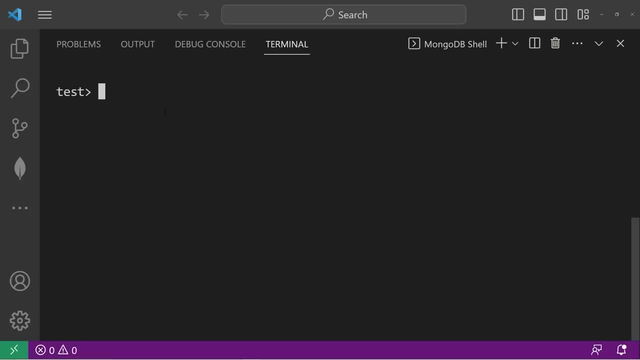 use databases in MongoDB To show all databases type: show DBS. That will give you a list of all current databases. I have three: admin, config and local. To use a database type: use Then select a database name. To use admin. I can say use admin. We have switched to DB admin Now if 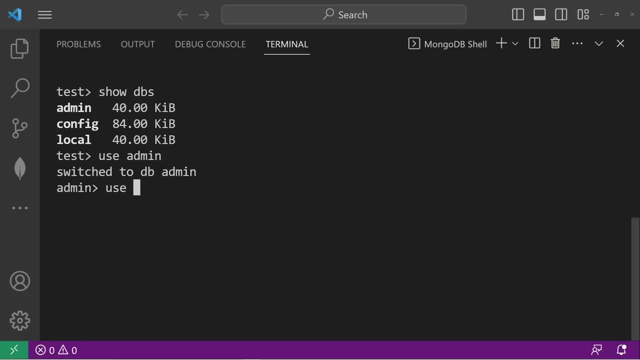 you use a database that's not an admin. you're not going to be able to use admin. You're going to have that doesn't exist. Let's say we will create a database for a school Use school. That's how you can create a database. We are now within a new database named school. However, 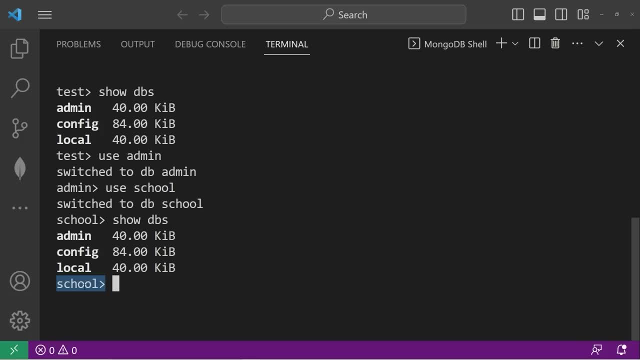 if I were to show my current databases. my school database doesn't show up. It's not visible because it's empty. We'll need to fill it with something. Let's add a collection to our school. To do that type db, We will use the createCollection method, This method. 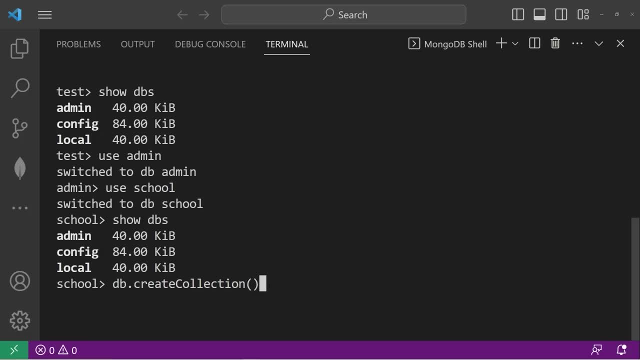 ends with a set of parentheses, just like a function or method in typical programming languages. Within the set of parentheses we are going to pass in an argument for a name for this collection. Let's create a collection of students We are returned with. OK, We have. 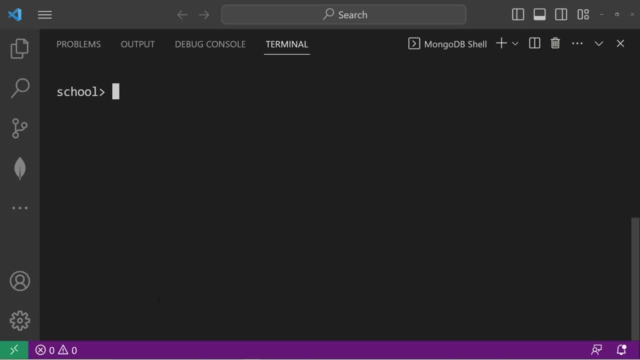 created one new collection. Let's clear our screen. Show our databases again, Show dbs. And here is our new database of school. Currently we are within our school database, as you can see. Next my cursor. To drop this current database, you can type dbDropDatabaseMethod And our 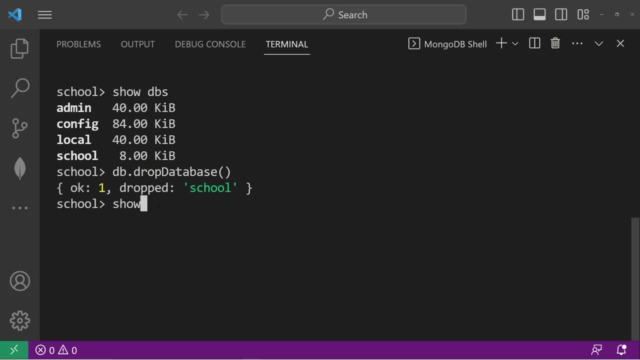 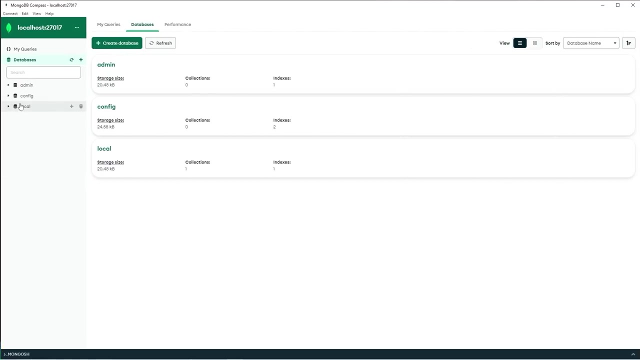 database is dropped, Let's show our databases again, And our school database is no longer there. That is how to use create and drop a database in the MongoDB shell. If you would like to use Compass, here's how We have our three default databases: admin. 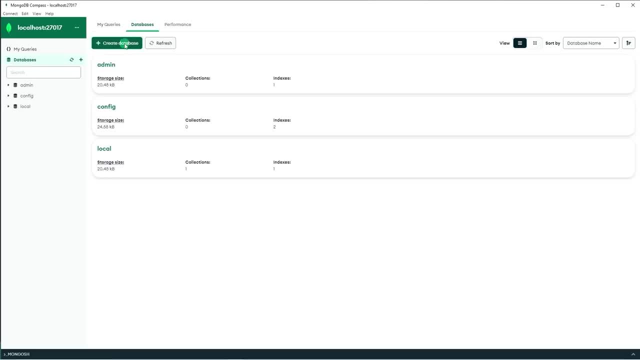 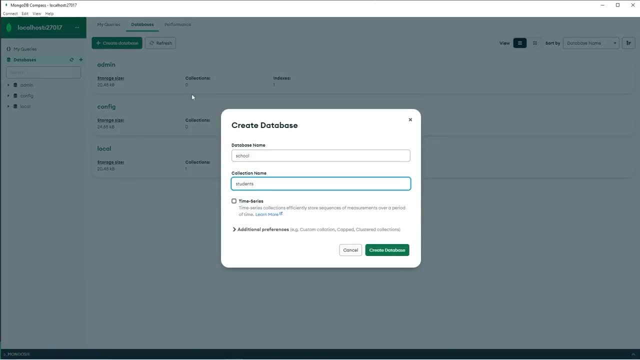 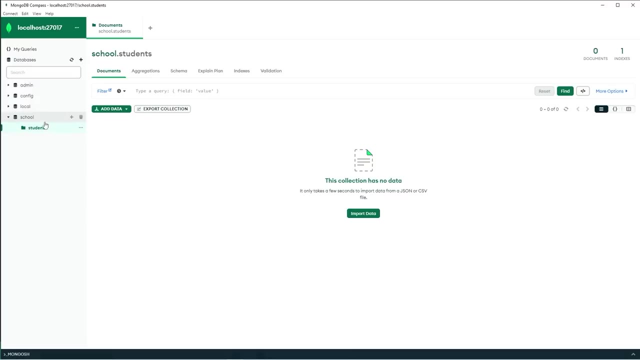 config local. To create a database, you can click this green button. We'll need a database name, Let's say school. again, We will create a collection of students within our database. You can add additional preferences, but we'll cover that later. We will create our database And here is. 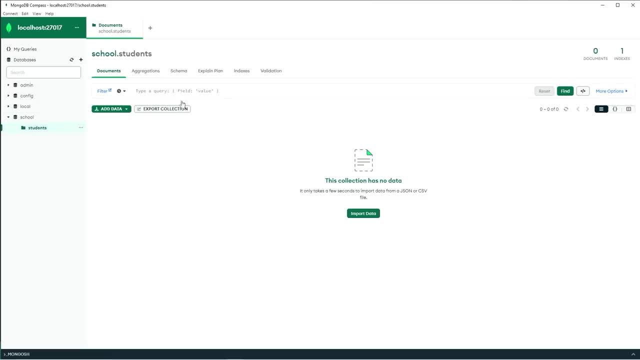 our database of school There is one collection of students, but students doesn't have any documents yet, which we'll cover in the next topic. To delete a database in MongoDB Compass: select a database from the sidebar, Then hit the trash can icon to delete it. Type the name of the. 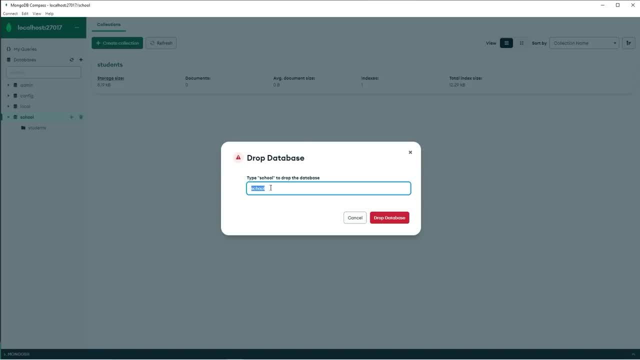 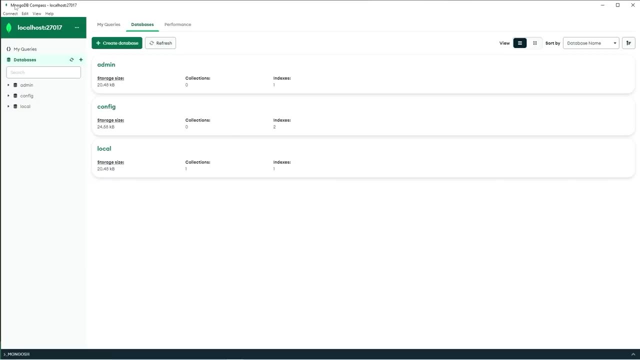 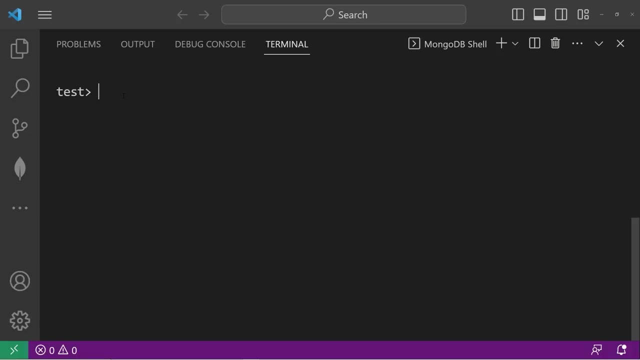 database, to drop the database. So make sure that the name of the database is typed, Then drop database. And that is how to use, create and drop a database in MongoDB Compass. All right, we're moving on, everybody. Now I'm going to show you how we can insert documents into a MongoDB. 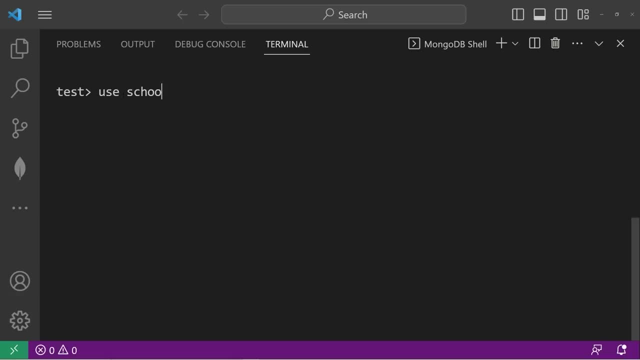 database. Let's be sure that we're using our current database. In the last topic we were using the database of school. Let's clear our screen To insert a document within the database. we're working with type db, then the name of a collection. if a collection is found within this. 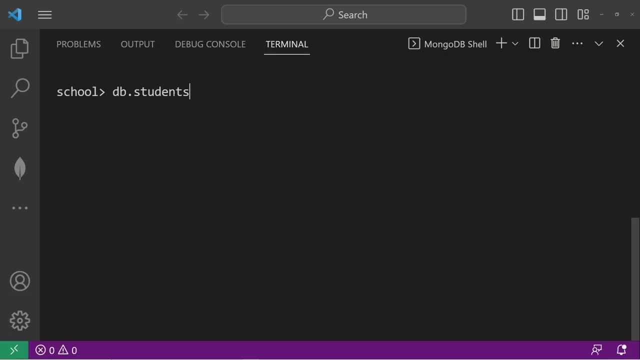 database. We have created a collection of students. If this collection doesn't exist, one will be created for you, dbstudents. We will use the insert, one method. Within the set of parentheses, we will place a document which is enclosed within. 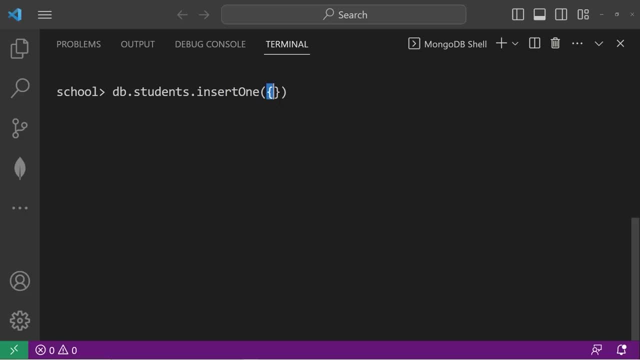 the set of curly braces. Within the set of curly braces we can list as many field value pairs as we would like. Let's create a name field with the value of Spongebob. Each field value pair is comma separated. Let's add another field value pair, Maybe an age. Age will be 30. Then a GPA grade. 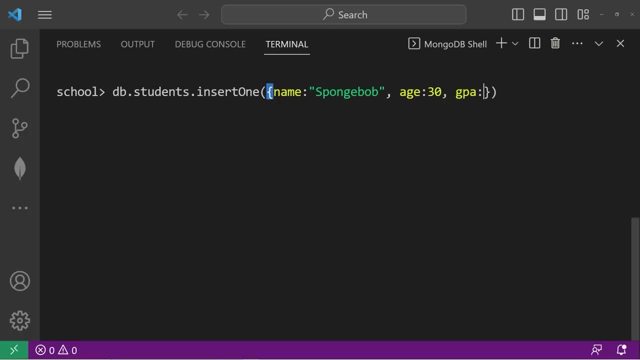 point average, Spongebob has a solid 3.2 GPA. Let's enter this command That was acknowledged To return all documents within a collection type: db: the name of the collection, in this case students dot. we can use the find method. Here are the: 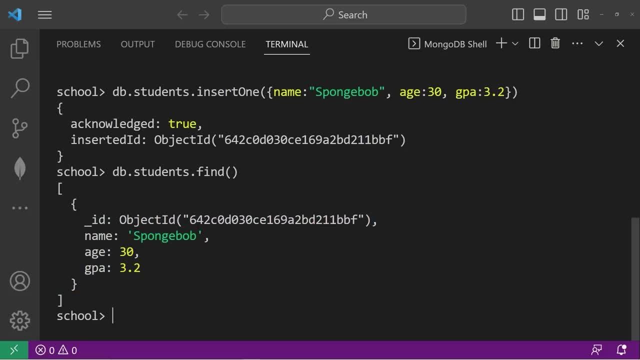 current documents within my collection, We only have one. Here's the object ID That's created automatically. The name is Spongebob, age 30, GPA 3.2.. Now you can insert more than one document at a time by using the insert many function. 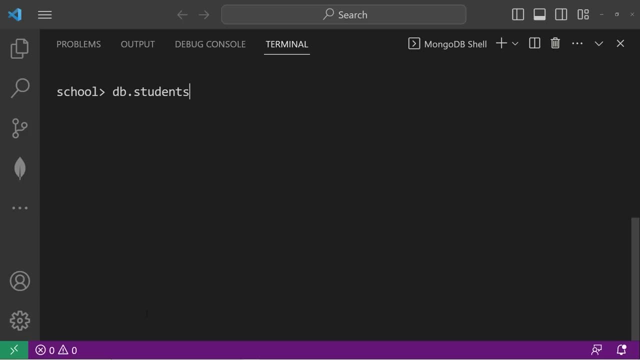 db type the name of the collection: students. in this case, We will insert many documents. We will place all documents to be inserted within an array, Add a set of straight brackets. This is the exact same kind of array from different programming languages. However, in Python I think that would. 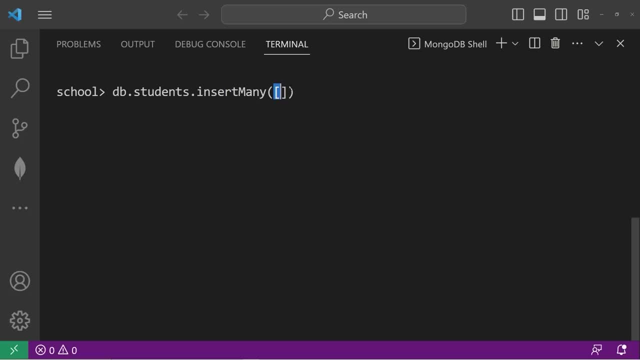 be a list. technically Maybe we need to insert three documents. We would need three sets of curly braces, each comma separated. Within each set of curly braces we would list all of three different field value pairs. Let's begin with the first. We have name Patrick. Separate each field value pair with a comma. Then we have 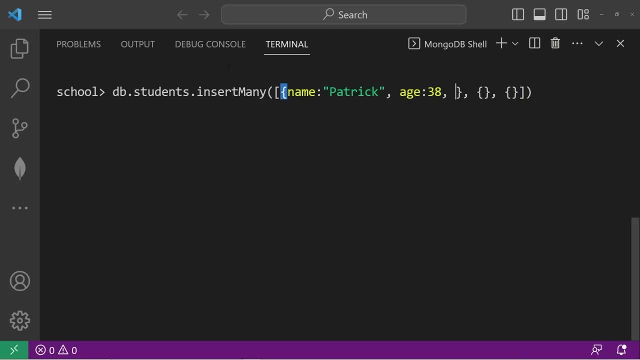 age of. let's make Patrick 38. Then GPA Patrick is at 1.5.. That's enough for our first documents. Let's go to the second document. move over to the second set of curly braces For the name. this will be Sandy. 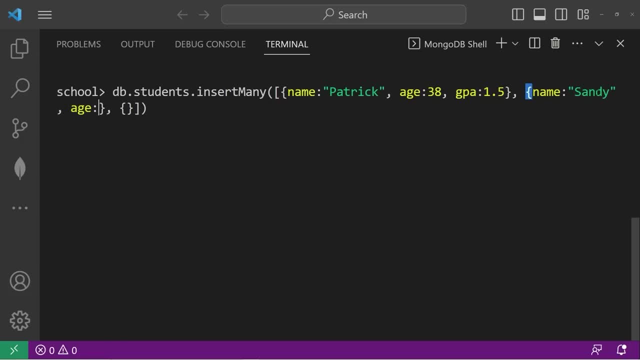 Sandy's age is, I don't know, 27 sounds good. GPA Sandy's smart. She has a solid 4.0.. Then let's go to the last document Name, maybe Gary. Gary's age is 18.. GPA 2.5.. That's good. 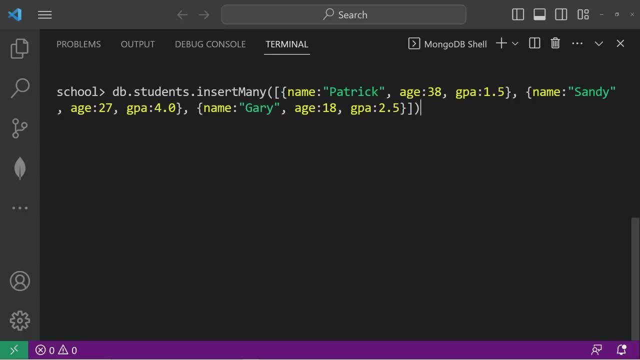 enough for now. This array contains several documents. Each document is enclosed within a set of curly braces. Within each document, you can have as many field value pairs as you like. They all don't need to be in the same set of curly braces. 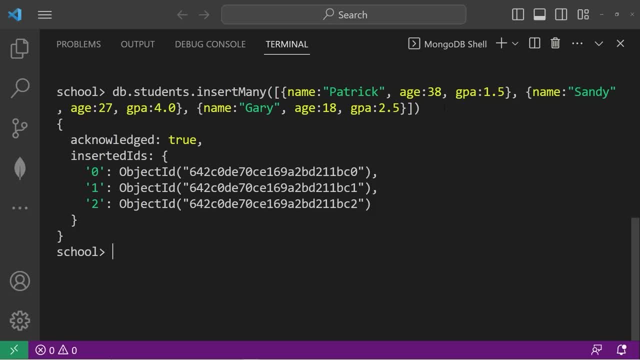 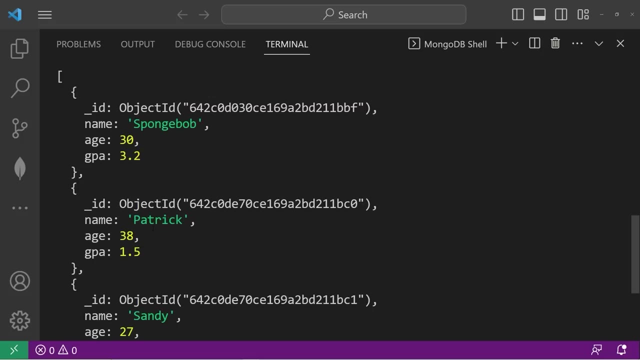 To be consistent, let's insert all of these documents. They were all acknowledged. We have three new object IDs. Let's use the find method again to display all of them: dbstudentsfind. Here are the four objects found within our database: Spongebob, Patrick, Sandy, Gary. 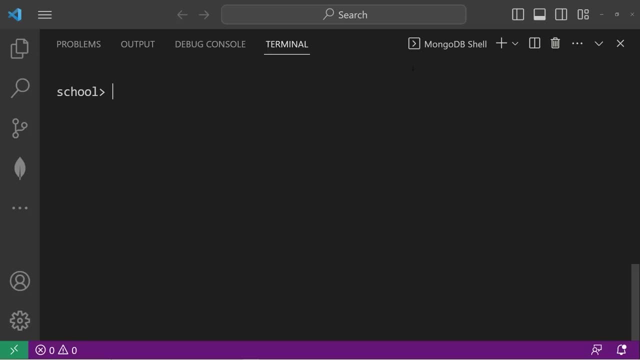 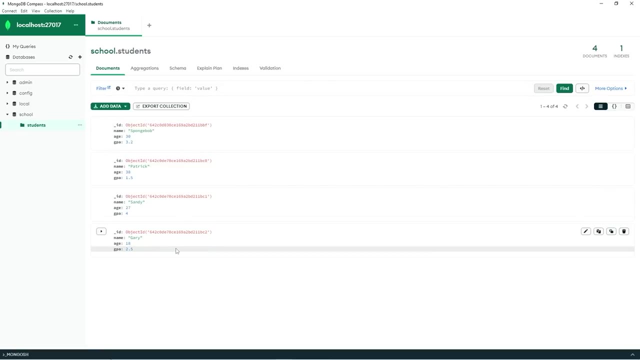 That's how to insert documents using the shell. Next, we'll do the same thing, but use Compass instead. If you're using Compass, here's how to insert documents into a collection. Here are the four documents. I'm just going to go ahead and delete these To add a new document. make sure you're within. 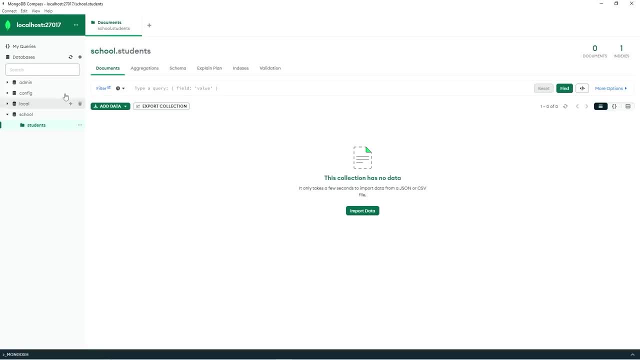 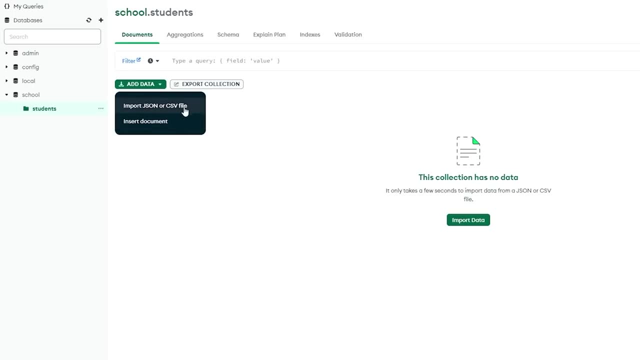 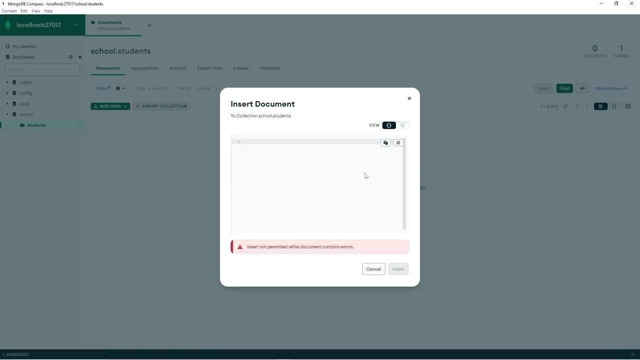 the current database you're working with. Go to the current collection. ours is students. We will add data. You can import a JSON or CSV file or you can type them manually by inserting document. A document is pre-generated for you. I'm just going to go ahead and delete that. 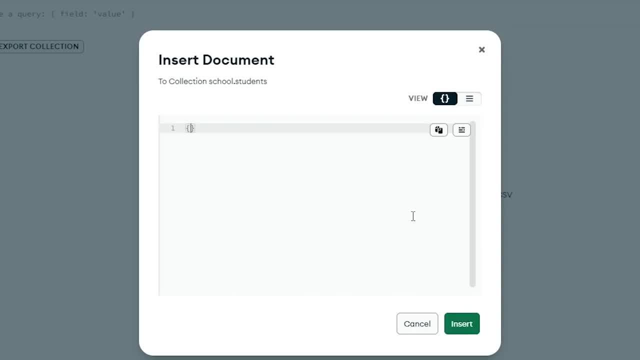 We'll begin by inserting Spongebob. You need a set of curly braces. then list all of the name value pairs: name Spongebob. separate each field value pair with a comma. age 30, GPA 3.2.. If you have this warning, you will need to probably hit the format button. 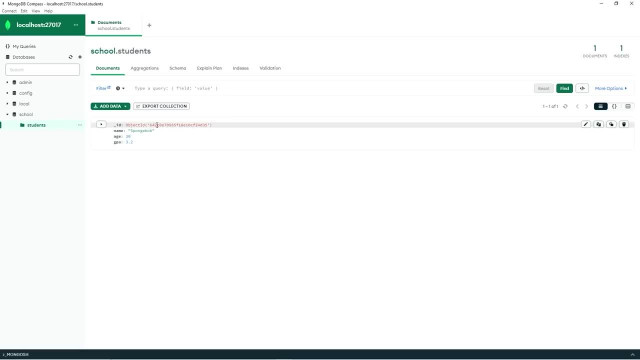 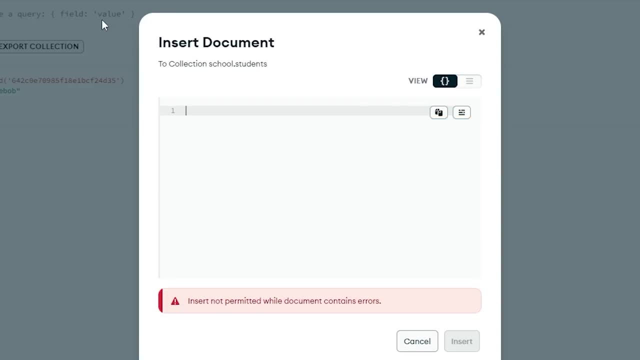 That should go away. Then insert. And that is how to insert one document, To insert many. it's the same process as before, But you're going to enclose all of your documents within an array, a set of straight brackets. So if we need three documents, 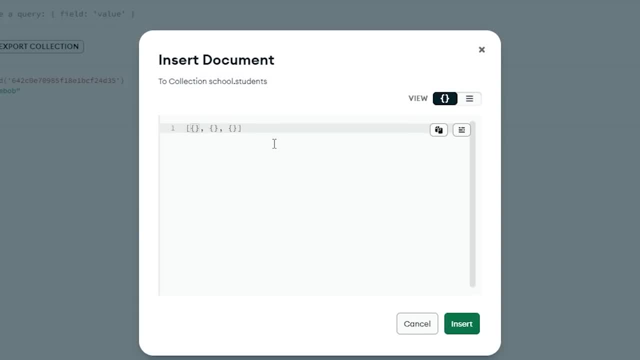 add three sets of curly braces, all comma separated. We had Patrick, Age I think he was 38. GPA 1.5. Name: Sandy, Age 27.. I'm going to move this down a little bit so you can see. 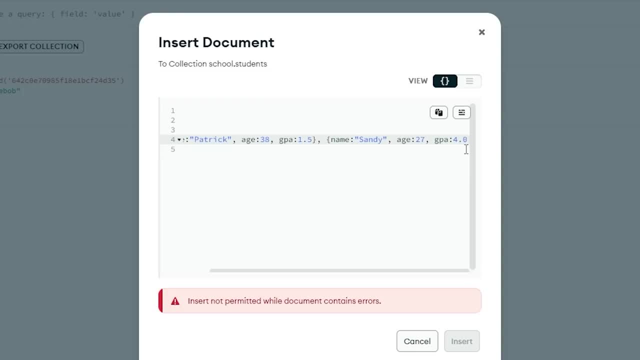 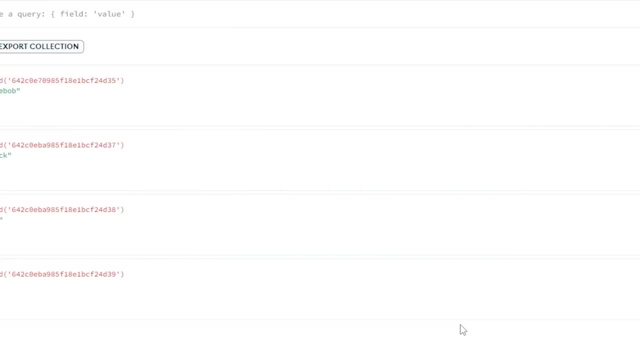 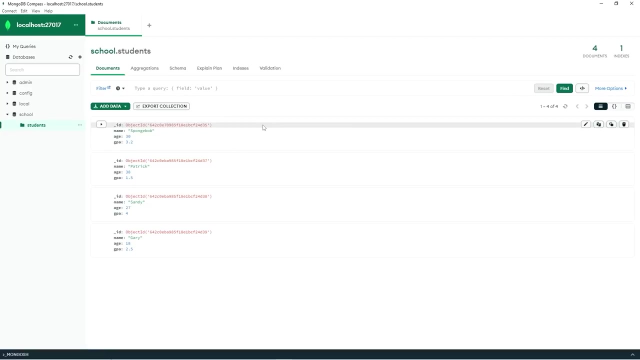 GPA 4.0.. Then name Gary, Age 18.. GPA 2.5.. Let's reformat, Insert And here are the three documents we have inserted. All right, and that is how to insert documents into a MongoDB database. 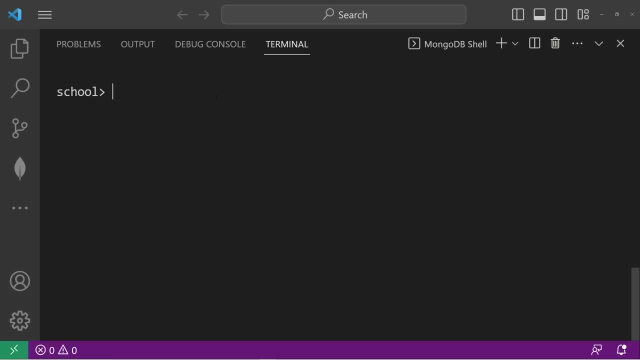 using Compass. All right, everybody, it's about time I discuss some basic data types in MongoDB. We will begin by inserting a new document into our students collection, dbstudentsinsert1.. We're inserting a document. add a set of curly braces. 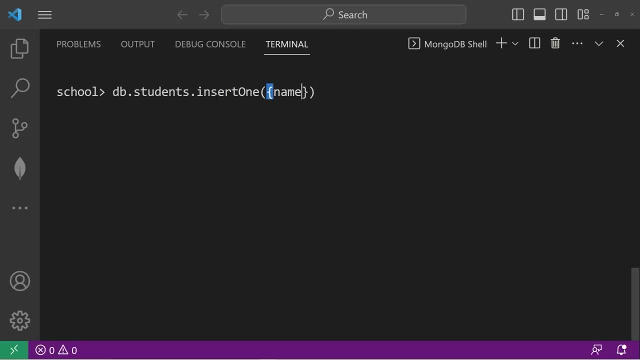 The first data type I'll discuss is a string. Suppose we have a field of name. A string is a series of text within quotes. These can be either double quotes or single quotes, but typically I like to put them within double quotes. A string is a series of text like a name, like Larry. 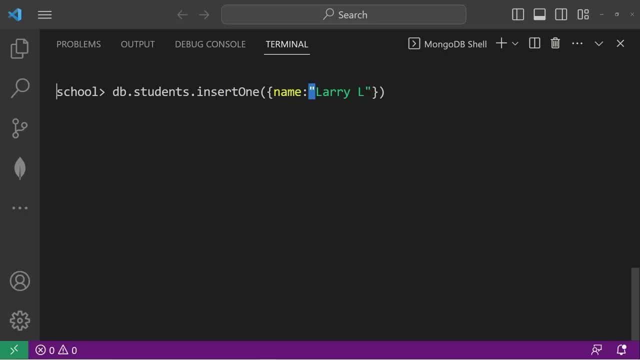 Strings can contain spaces. We can enter in a first name space, then a last name: Larry Lobster. They can also contain numbers: Larry 1,, 2, 3.. However, in a string we treat the numbers. 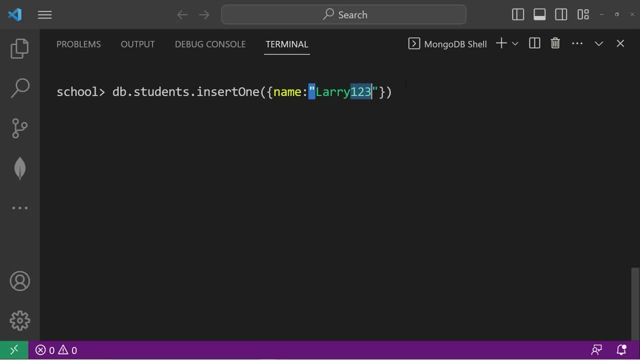 differently. We read them more as characters rather than actual numbers. So let's stick with name Larry, That's a string, It's a series of characters. Then we have integers. An integer is a whole number. Let's create a field for age. Larry will be. 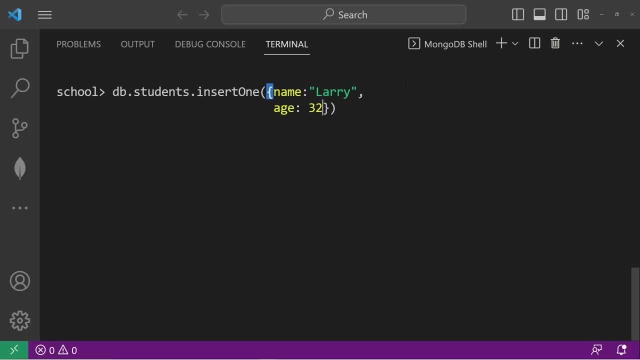 32. Whole integers don't contain decimal portions. It wouldn't make sense to enter in 32.5.. We don't really keep track of people's half birthdays and stuff, So age would be a whole number. Those are integers, whole numbers. Then we have doubles. A double is a number that contains a. 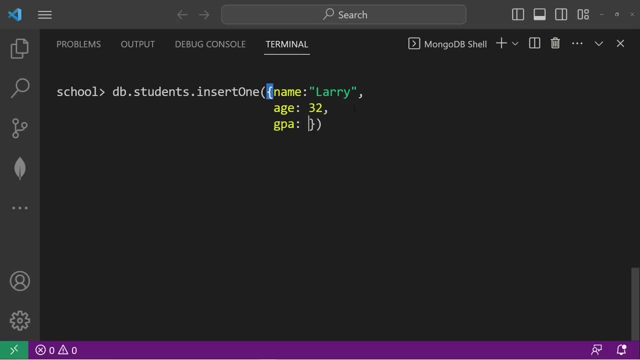 decimal portion, Maybe a grade point average. Grade point averages typically contain decimals. Larry has a 2.8 GPA because there's a decimal portion. Integers are whole numbers. Doubles are numbers that contain a decimal. Then we have booleans. Booleans are either true or they're false. It's kind of like. 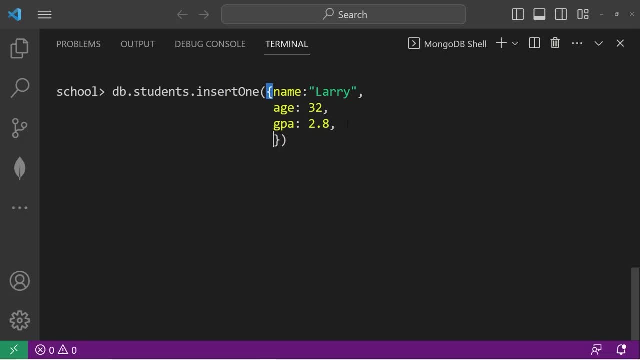 a light switch. It's only on or off. There's only two states. Let's create a field for full time. Is the student full time? This can be either true or false. Larry is too busy working out all the time. He is a part-time student, not a full-time student. We'll set that field to be false. 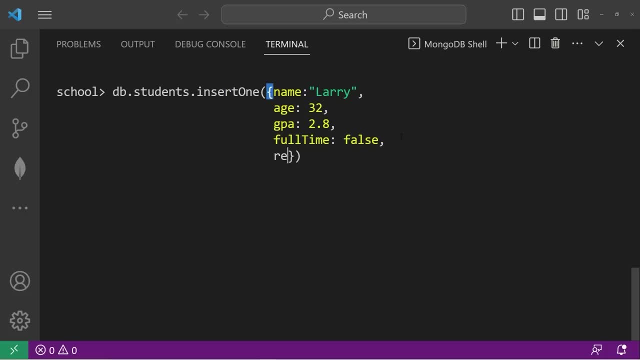 Date objects are pretty popular in MongoDB. Suppose we have a registration date, Register date. To create a date object, you can use the new keyword, followed by a call to the date constructor. If you don't pass any arguments to the date constructor, you'll use the current time. 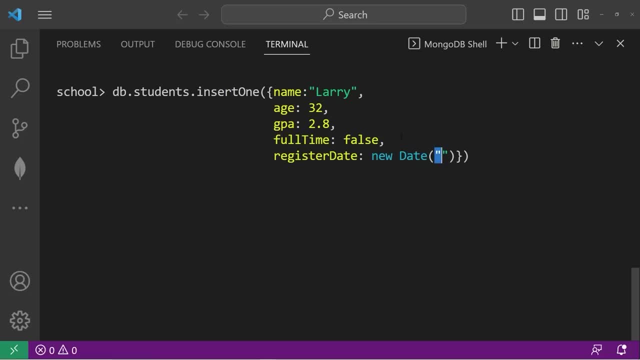 in the UTC time zone. Otherwise, you can pass a date and time like 2023, January 2nd. You could add a time too, but we'll just stick with the current date and time that's assigned to us. Those are date objects. The next data type is null. Null means no value. I'll create. 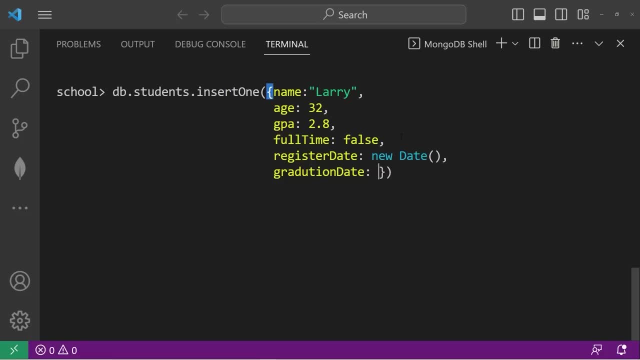 a field for a graduation date and I will set that to be null. Larry is a current student, but we don't know when he's going to graduate. All we're really doing is creating a placeholder. We don't have a date yet, so we can set that to be null. 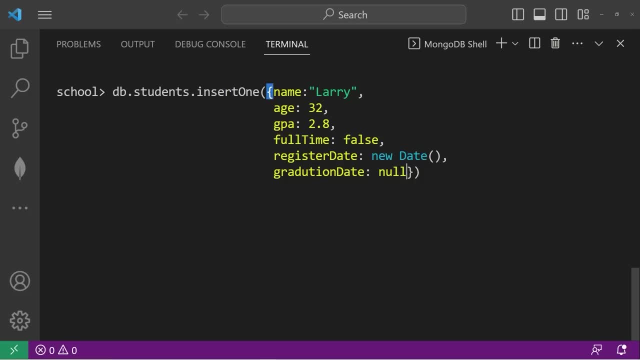 That's to be filled in later. So null means no value. Then we have arrays, Much like in modern programming languages is kind of like a variable that has more than one value, But in MongoDB we have a field that can have more than one value. Let's create a field of courses. What courses is? 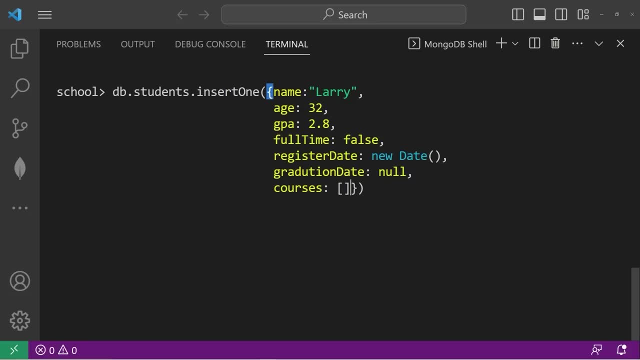 Larry enrolled in Place all values within a set of straight brackets. Let's insert multiple values. What courses is Larry in? Maybe he's in Biology? These values are all comma separated: Chemistry, then Calculus, So that's an array. They're all enclosed within a set of square brackets. 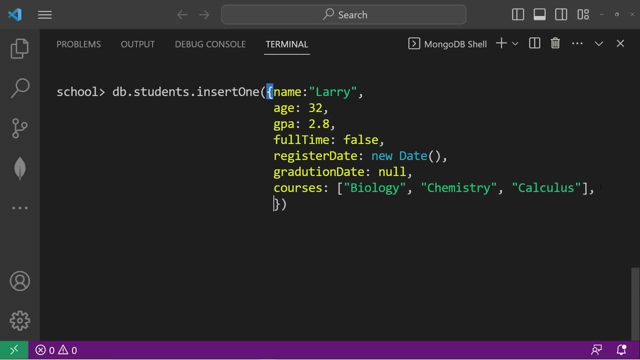 They allow one field to contain multiple values. Then we have nested documents. This would be good for an address. To create a nested document, you use a set of curly braces. Within the nested document we can list nests and values. Within the nested document we can list some field value pairs. 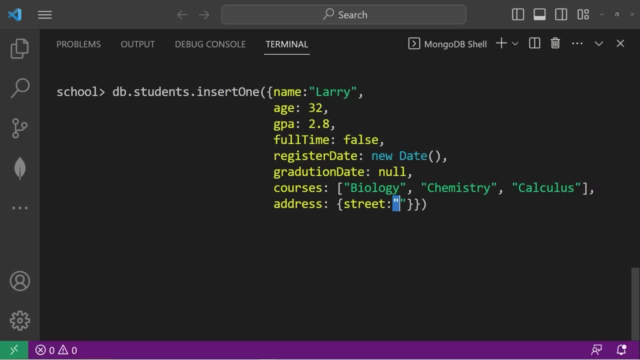 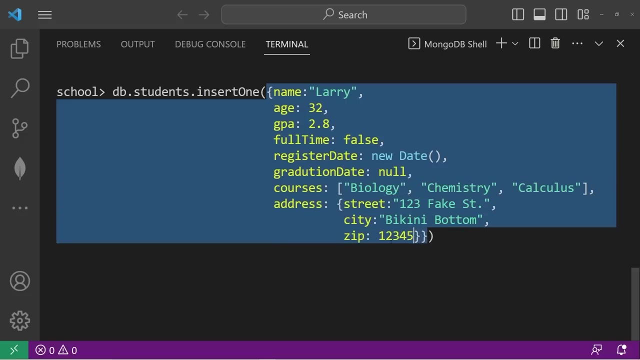 How about a street? Let's come up with a street name: 123FakeStreet is good. Then a city, BikiniBottom, and a zip code: 12345.. It is possible to have documents within documents, which is what we did with the address. 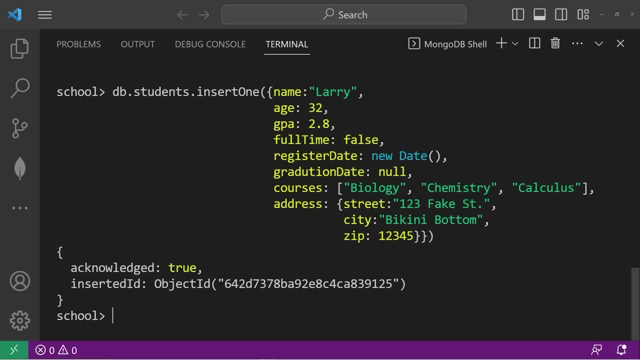 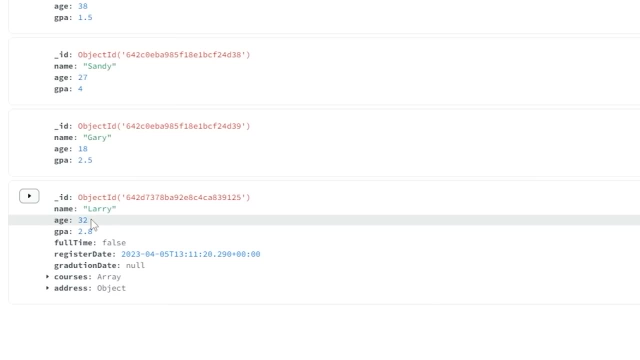 Let's enter everything to see if it works. Yeah, that was acknowledged. Let's head to Compass refresh. and here is Larry. Name: Larry, age 32, GPA 2.8.. Full time is set to false. he's a part time student. 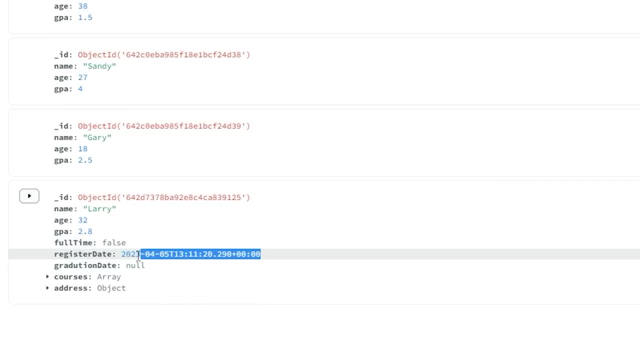 Here is Larry's registration date and time. We're using the UTC time zone. His graduation date is set to null. All of his courses that he's in- All of his courses that he's in- is stored within an array And his address is stored as a nested document. 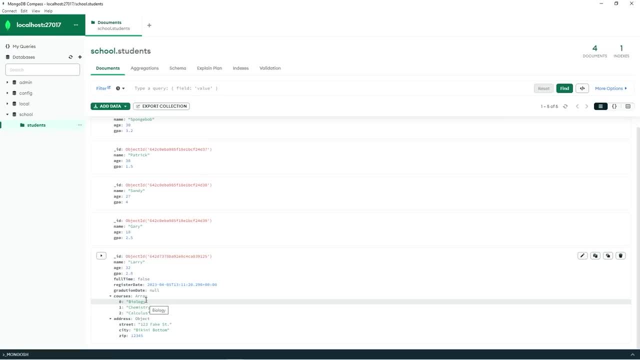 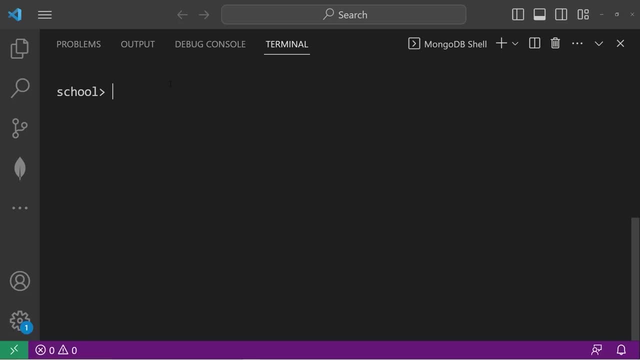 All right, everybody. and those are a few basic data types you should know in MongoDB. All right everybody. today I'm going to show you how we can both sort and limit documents in MongoDB. To return all documents we can type db- the name of the collection, dot. then we can use 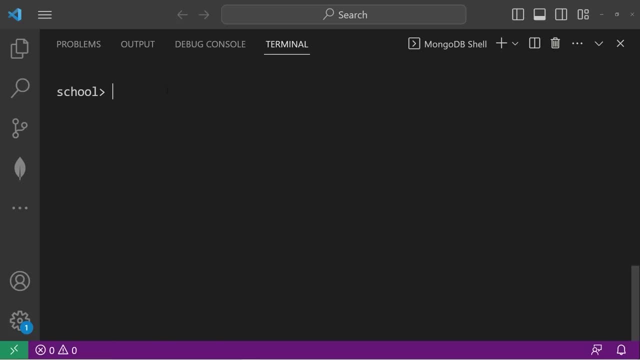 the find method to return all documents. To sort these documents in some sort of order again, we would type db- the name of the collection, students dot. find method. Then we'll do some method chaining. After the find method: add dot. then we will call the sort method. 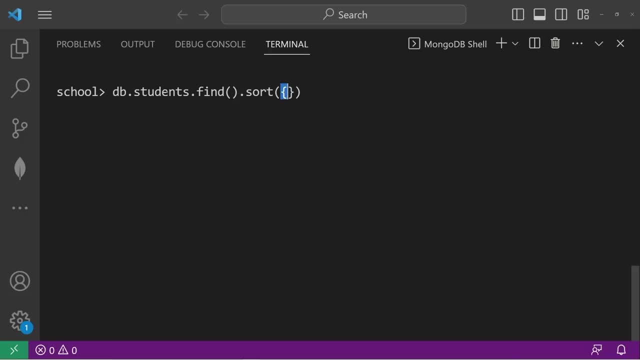 The sort method takes a document. By which field would we like to sort? Let's sort names in alphabetical order. We would type the name of the field, name colon, then one for alphabetical order or negative one for reverse alphabetical order. 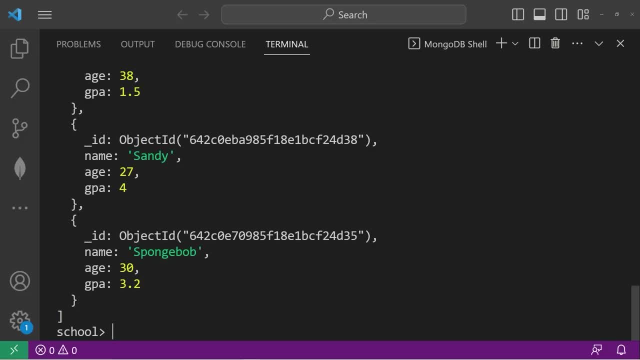 So if we were to sort by alphabetical order, here's the results. We have Gary, a student, dot dot. We have Gary, then Larry Patrick, Sandy SpongeBob. Then reverse alphabetical order. that was name colon negative one. 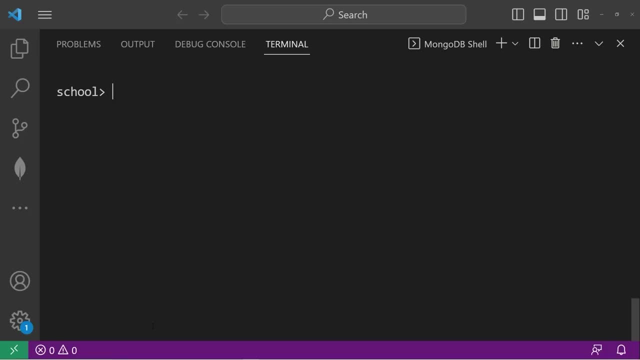 Now we have SpongeBob, Sandy, Patrick, Larry, Gary. Let's sort our documents by GPA grade point average. So again, we use the find method, then we'll method chain the sort method We're passing in a document object with our criteria. 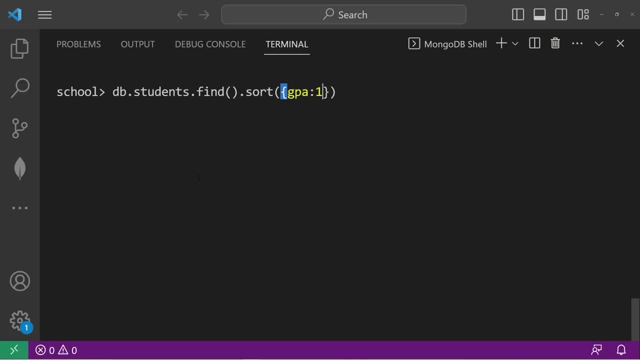 We will sort by GPA in ascending order, so we will use one. I'm going to copy this because I'm going to use it later. Now we're sorting by GPA. Patrick has the lowest GPA: 1.5,, 2.5, 2.8,, 3.2, then 4.. 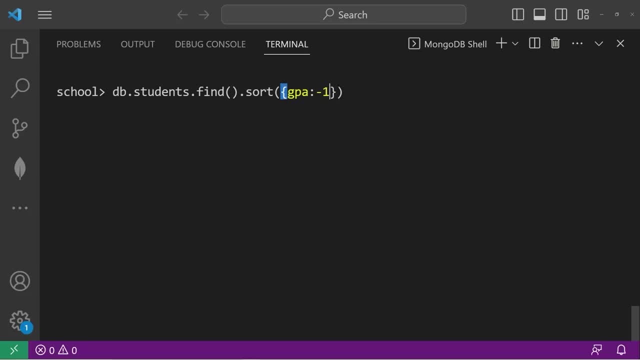 To sort our GPA by descending order, we would type GPA negative one, Then we have Sandy at the top with the GPA negative one, Then we have Gary the student dot dot dot. Then we have Gary the student dot dot. 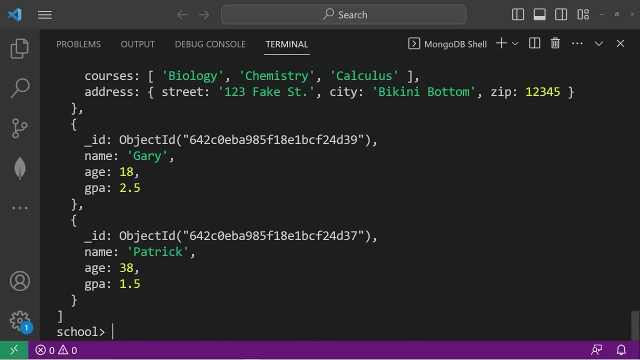 Then we have Gary the student dot dot, Then SpongeBob with 3.2, 2.8,, 2.5,, 1.5.. Now we have the limit method. We can limit the amount of documents that are returned to us. 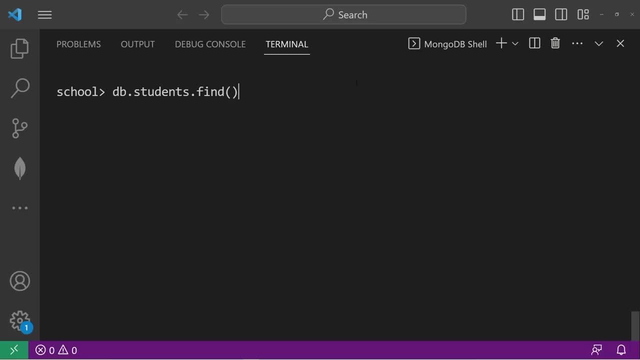 Let's type db, dot, students, dot. find method, dot limit method. We will pass the number of documents we would like returned to us. as an argument, If I would like one document returned to us, I will pass in one. 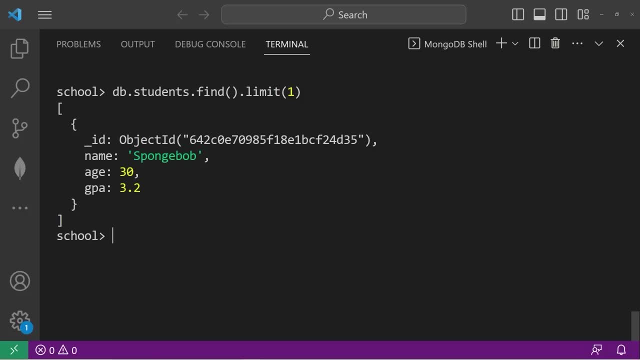 Currently my documents are sorted by object ID. This would give us the first document of SpongeBob. If I were to use limit three, we would be returned three documents: SpongeBob, Patrick, Sandy. We can combine both the sort and the limit methods too. 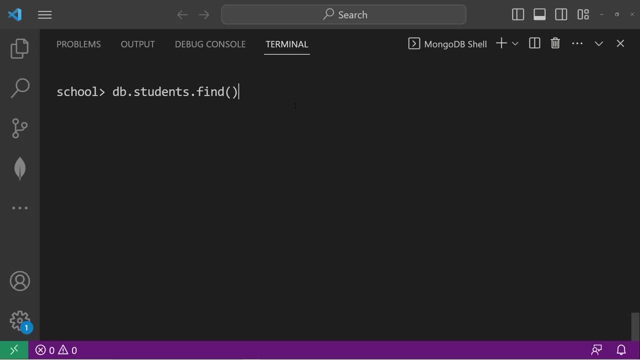 I would like to return the student with the highest GPA. We'll use the find method, then method chain, the sort method We are sorting by GPA. We're going to sort in decreasing order, So negative one, Followed by the limit method. 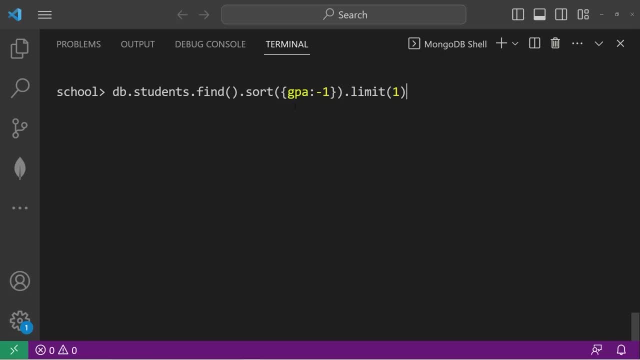 I would like just one document. Who has the highest GPA? That would be Sandy, with a GPA of four. Who has the lowest GPA? We should sort in increasing order. That would be one, then limit one. So Patrick has the lowest GPA of 1.5.. 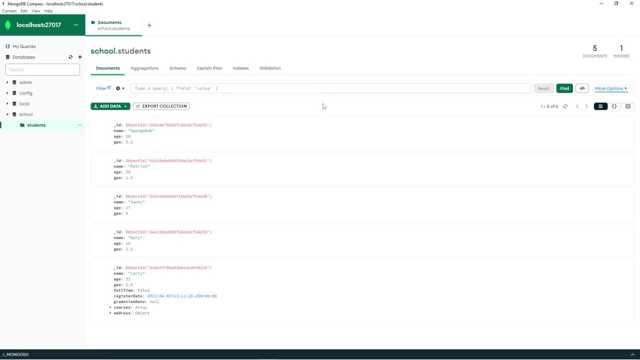 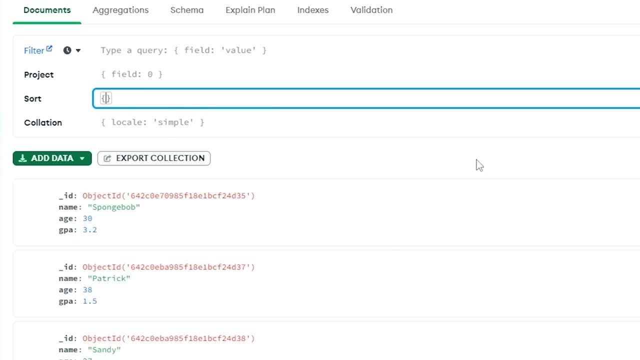 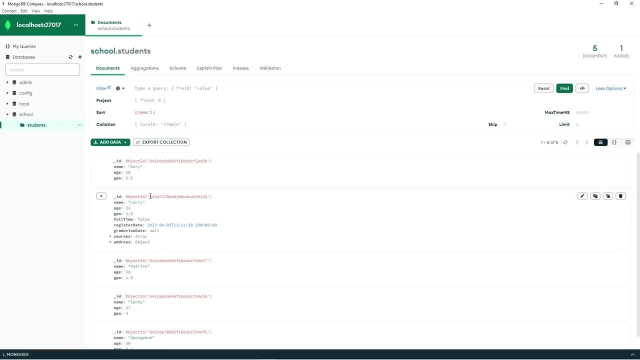 Now let's work with sorting and limiting in Compass To sort the documents in your collection you can press more options, Then add some sort criteria. I will sort by name, Name, colon one, Then find: So we have Gary, Larry, Patrick, Sandy, SpongeBob. 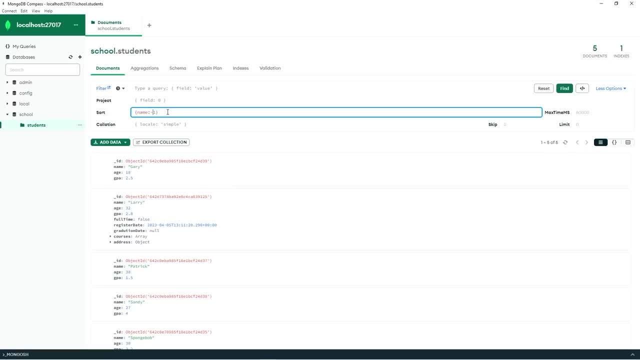 Then negative one. for reverse alphabetical order: SpongeBob, Sandy, Patrick, Larry, Gary. Let's sort by GPA: GPA: negative one. That would give us decreasing order. So Sandy's at the top To limit the amount of documents that are returned. 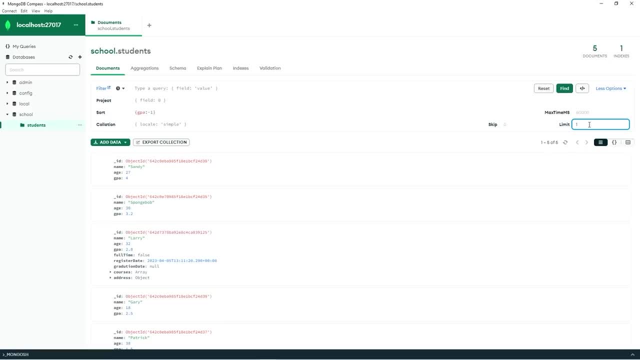 you can enter in a number for the limit box. I will limit the records to one. So we are returned with Sandy. She has the highest GPA. Limit three would give us the top three students. Or leave limit empty to return all documents. 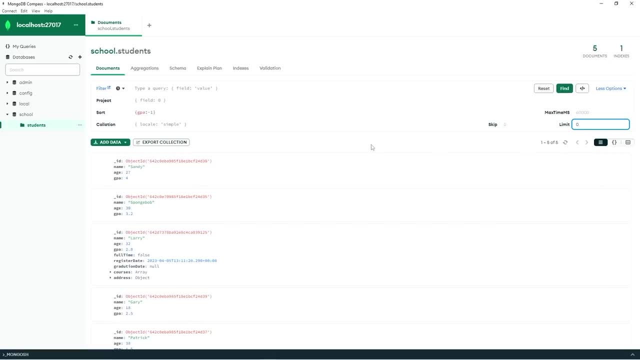 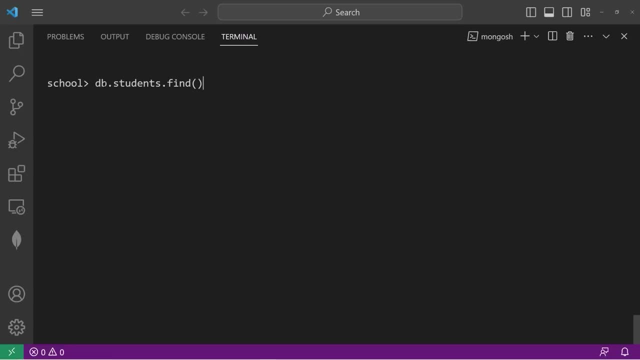 All right, everybody. So that is basic sorting and limiting in MongoDB. Hey everybody, In this topic I'm going to explain the find method in MongoDB. To use the find method type DB: the name of the collection you're working with. 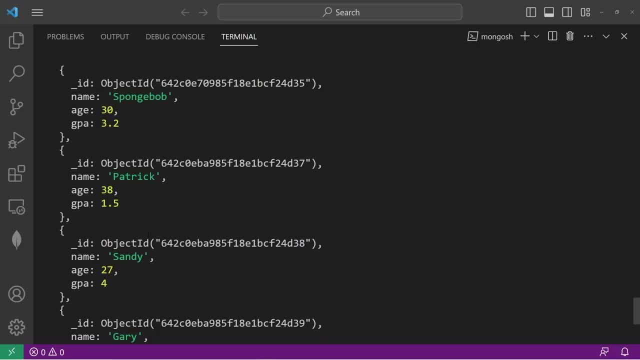 then add the find method. That will return all documents within this collection. But at times you might not want all documents. You might want specific documents. Here's how We will add some arguments to the find method: DBstudentsfind. The first argument is a document object. 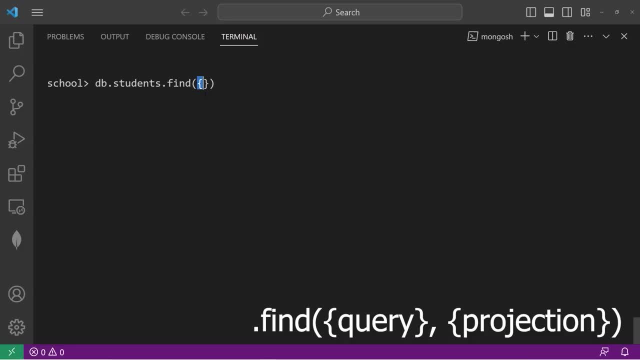 The parameter is the query parameter. It specifies selection filters. Maybe you just need one student. Well, you would just list that criteria here. I would like Any students with the name of SpongeBob. That would return any document where the first name is SpongeBob. 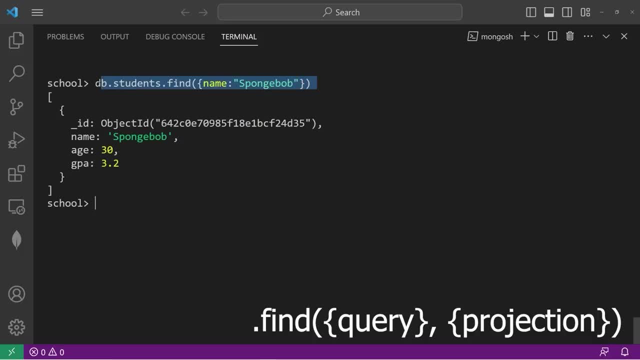 That would return everybody that has that name. I'm just going to copy this: Let's find any students that have a GPA of 4.0. Within our document, the search filter is GPA 4.0.. That would give us Sandy. 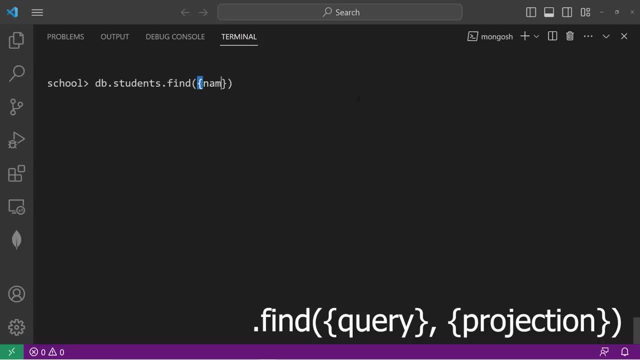 Let's find if any students are not full time- Full time- I will set that to be false. There is one student, Larry. full time- is set to false. The query parameter is very similar to a WHERE clause in SQL. You can even use more than one filter. 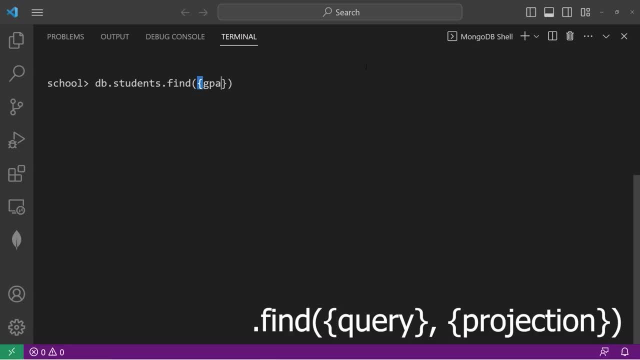 Search for any student that has a GPA of 4.0.. Each filter is comma separated. As well as full time being true With my data set, this does not return any results. But to add more than one filter, they're comma separated within a document body. 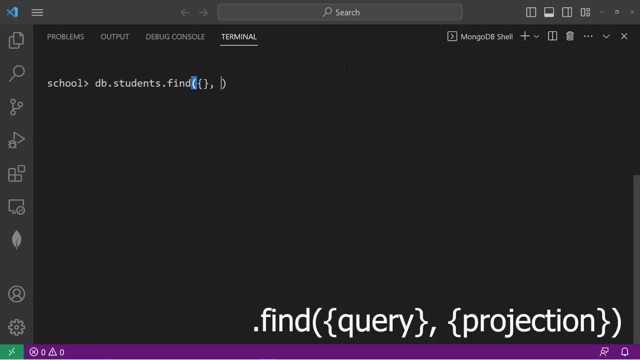 With the find method. there is a second parameter, That is the projection parameter. We would pass another document body. They're each comma separated. If you don't specify the query parameter, you would just return all documents. With the projection parameter you can return specific fields. 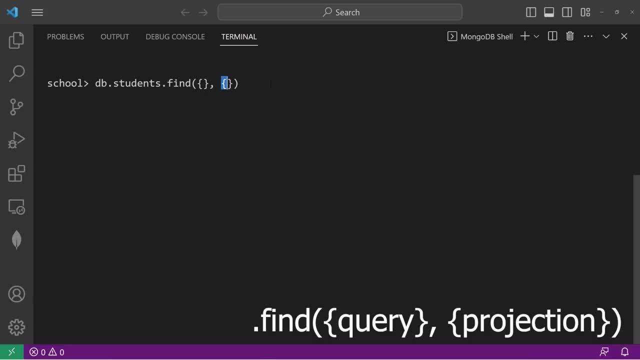 Maybe you don't want all the information that's available. Perhaps I would just like Each student's name, So we would set the field to be true. You can use one as well, But my own preference is true, Just because it's more readable. 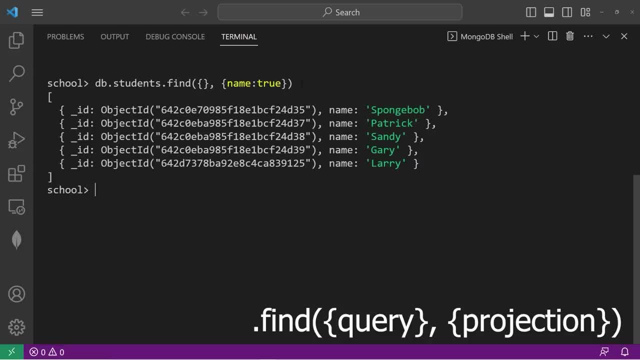 Return every document, But only give their name. And here they are. MongoDB will give you the ID regardless. You can set that to be false Within the projection parameter. Underscore ID False. I just want everybody's name. 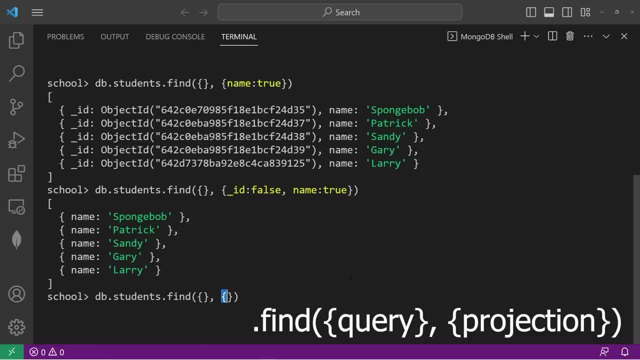 There we are: Rick, Sandy, Gary, Larry. Let's get every student's name as well as their GPA, So ID. I will set that to be false. I don't want that Name will be true. I would like that. 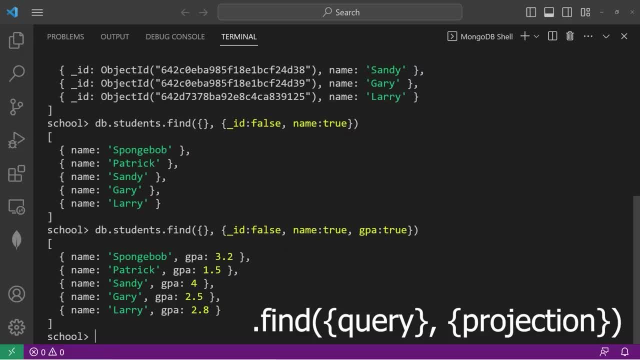 GPA will also be true. I would like that. Here is every student's name as well as their GPA, So that's the projection parameter. If there's a field you would like or don't want, you can set that to be either true or 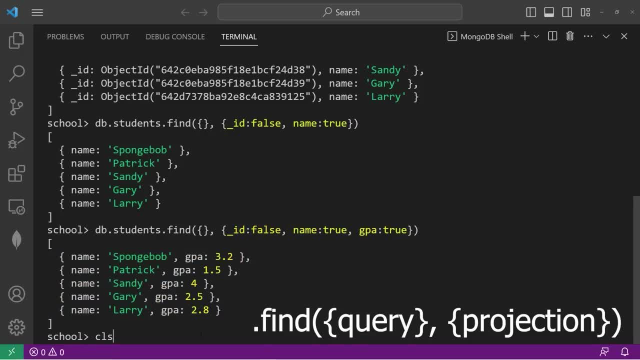 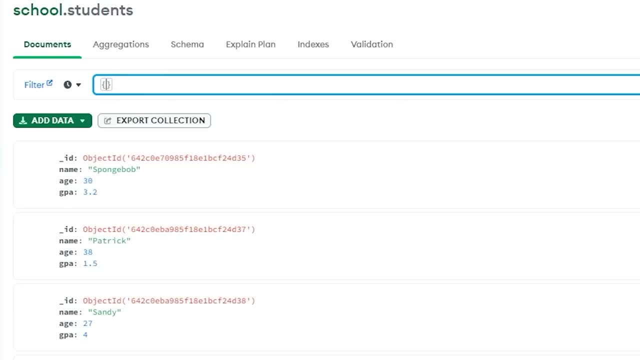 false when you display your data. All right, Let's do the same thing with Compass. With Compass, this text box is for the find method. So within a set of curly braces, I would like to find any name, that's SpongeBob. 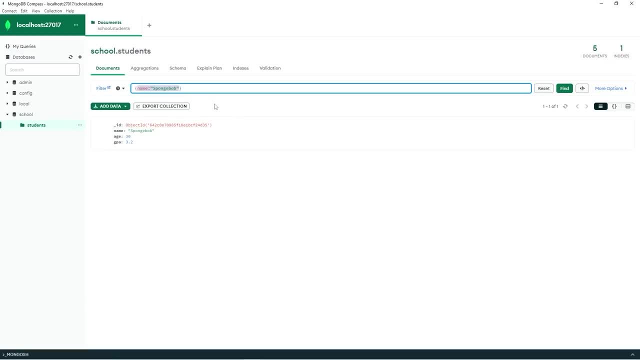 Then press find. That returns one result: Return any student with a GPA of 4.0. That's Sandy. Return any students that are not full time. Full time is false. That gives us Larry. Now, if you go to more options, there is a projection parameter. if you only want some, 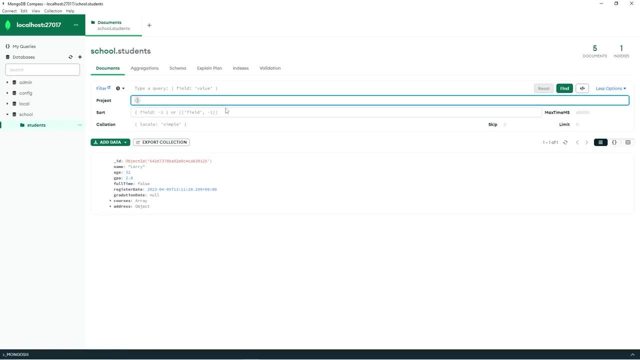 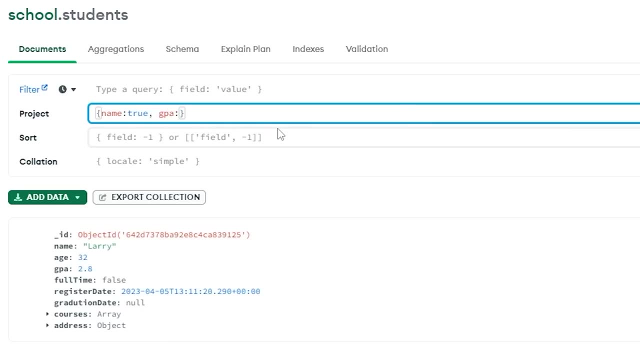 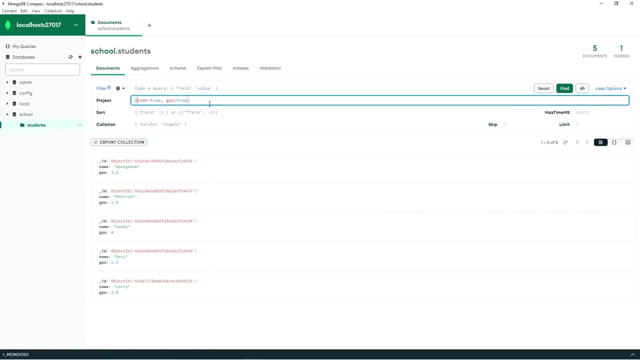 data. Let's find every student, but for the projection parameter, I would only like their name- I'll set that to be true- And their GPA- That's true as well. Again, that still gives us the ID. Let's set that to be false if you don't want that. 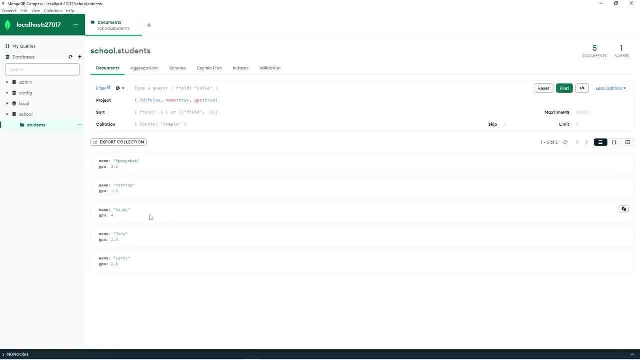 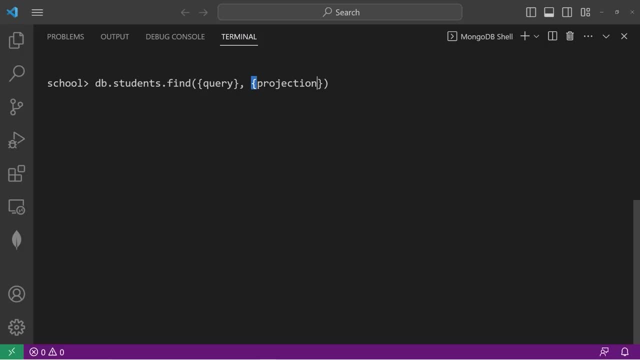 ID False And that should get rid of the IDs. Here's each student's name and their GPA. All right, everybody. That's the find method. Two optional parameters that we can send arguments to are the query parameter, That's selection criteria. 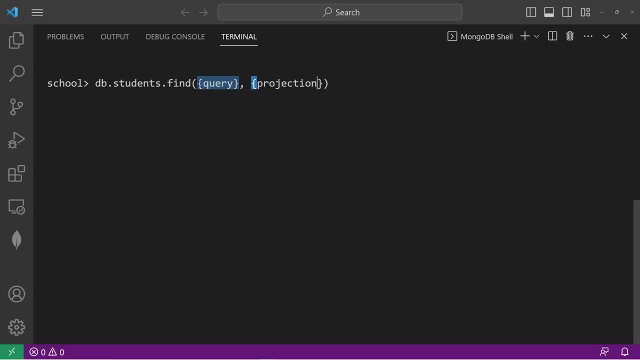 It's similar to a where clause in SQL. We're trying to limit the results And the projection parameter. that's similar to selected columns in SQL. You're looking for specific fields. All right, everybody, And that is the find method in MongoDB. 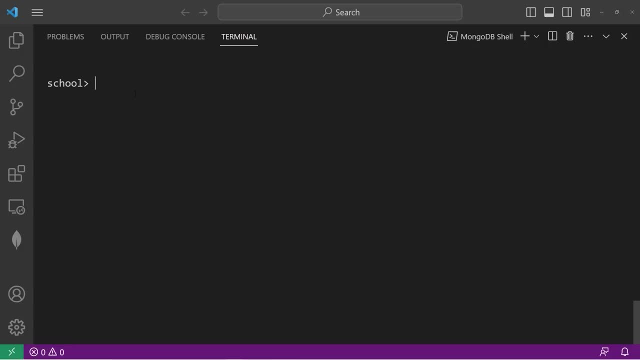 Well, hello again everybody. Today I will be explaining how we can update documents in MongoDB. To do that, we would type db- the name of the collection we're working with, in this case students. We can either update one document or update many. 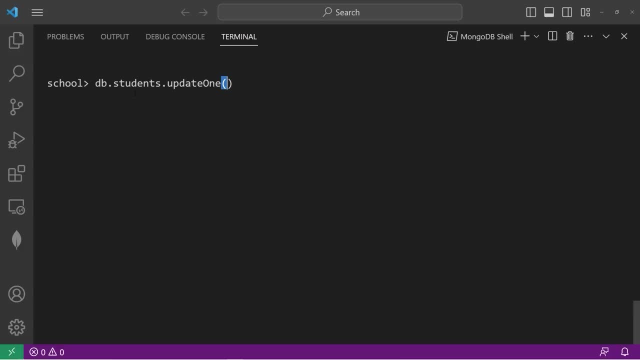 Let's update one. We will use the update one method. There are two parameters: set up Filter and update. Filter is the selection criteria for the update. So within a set Of curly braces, we will pass some criteria. Let's update anybody's name. 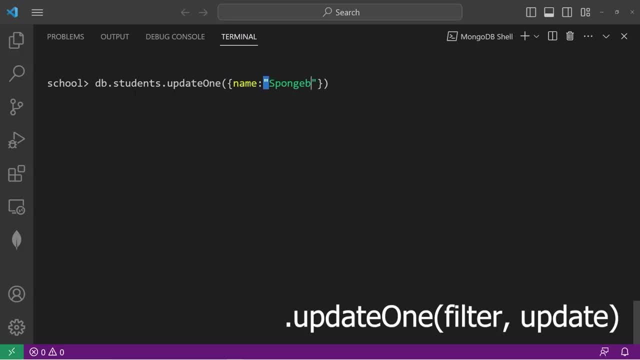 That's SpongeBob. It's basically just selection criteria. The second parameter- it's another document body- is the update parameter. What are the modifications we would like to apply? We will utilize the set operator, which is preceded with the dollar sign. 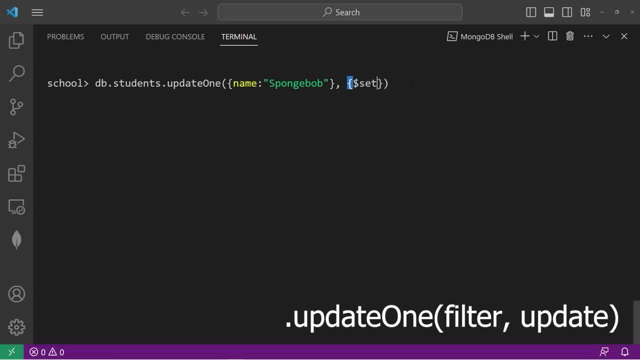 The set operator. It replaces the value of a field. So after the set operator, add a colon. Then another set of curly braces. Yes, there's a lot of curly braces in MongoDB. So within this set of curly braces after the set operator, that's where we can make. 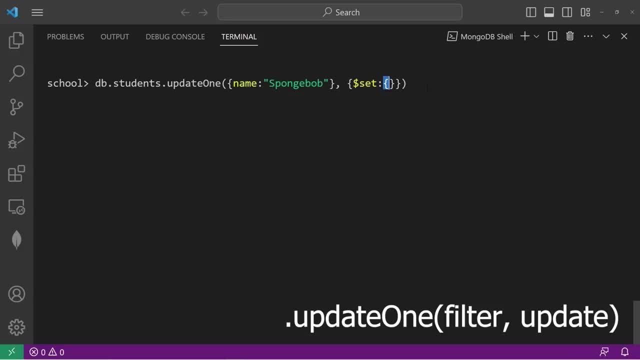 our changes. You can add or change the value of a field. SpongeBob doesn't have a full time field. We can add that with the set operator. If this field already exists, we would update it. So let's say SpongeBob is a full time student. 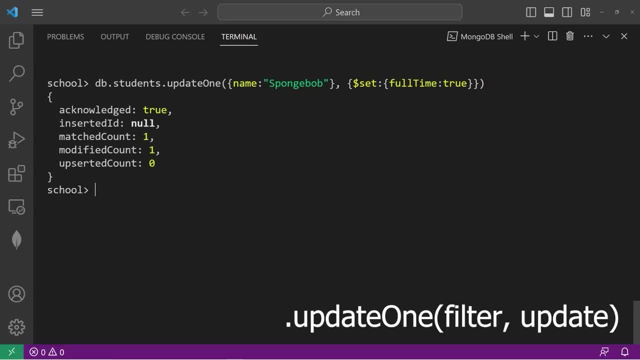 Let's execute this command. It was acknowledged, That's true. We have a matched count of one and a modified count of one. Let's take a look at SpongeBob: dbstudentsfind name SpongeBob And here he is. He is now a full time student. 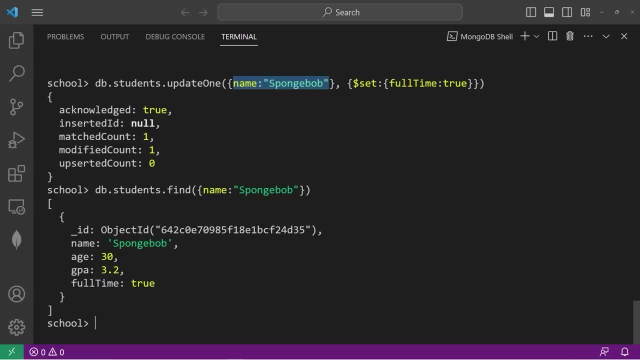 With your filter argument. if you're working with a large data set, it is possible that two people can have the same name. It would be safer if we were to update by an object ID. These IDs are unique for each document. Let's update. 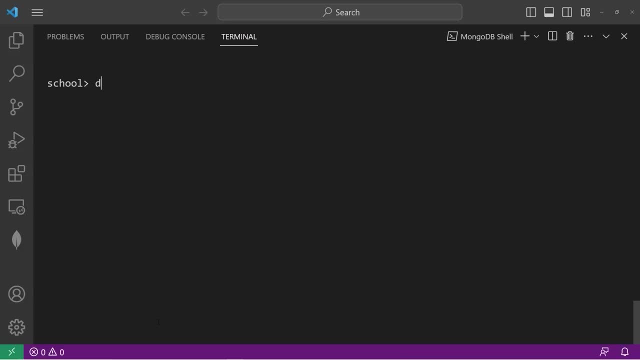 But with the filter we will search by object ID. So again, that's dbstudentsupdate1.. First is the filter parameter. within a document body, Let's select underscore ID colon, then paste that object ID for SpongeBob. For every document the object ID is unique. 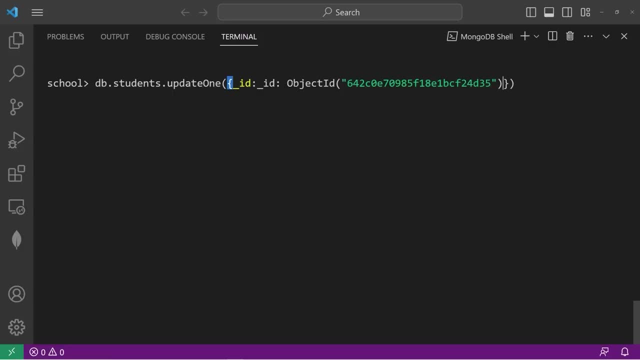 Just in case there's two people named SpongeBob. we won't update it. Looks like I have double underscore ID. Let me fix that real quick, Otherwise we'll get a syntax error. So select the document that has this object ID. Then the second argument, which is comma separated, will be the changes to be made. 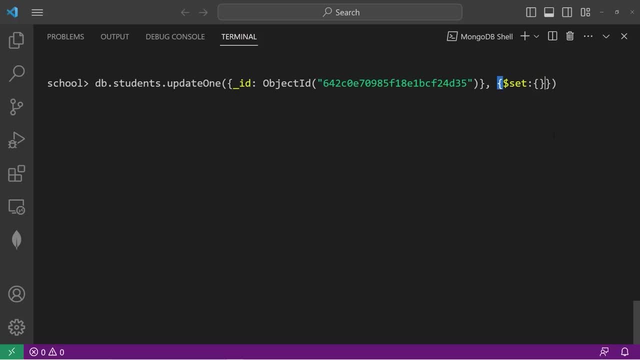 So we will set colon: another set of curly braces. Let's set full time to be false, SpongeBob already works a full-time job. He'll just be a part-time student. Okay, that was acknowledged. Let's take a look at SpongeBob again using the find method dbstudentsfind ID colon. 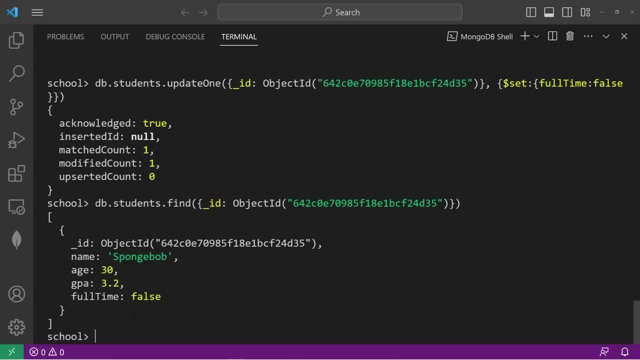 the unique object ID, And here's SpongeBob. The full-time field is set to false. Before it was true, but we updated it. Now. you can unset a field too. Let's get rid of the full-time field for SpongeBob. 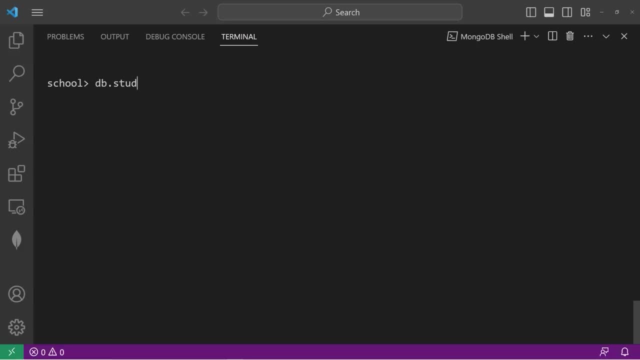 Let's get rid of the full-time field for SpongeBob- dbstudentsupdate1.. We will search by ID. Then, for the second argument, we will use the unset operator, which will remove a field. So, within another set of curly braces, let's take our full-time field colon. 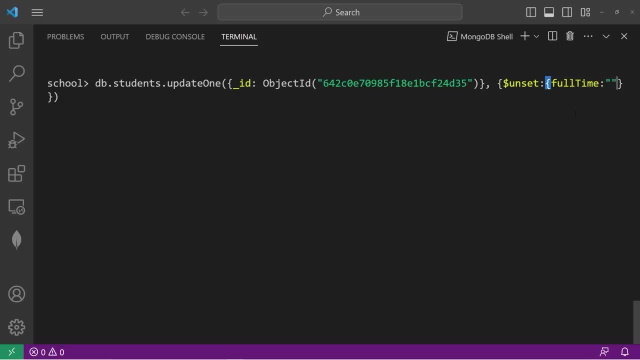 Now to remove a field for the value, just set it to be an empty string. Let's take a look. That was acknowledged. Let's select SpongeBob again- dbstudentsfind. Alright, and here's SpongeBob again. That full-time field is gone now. 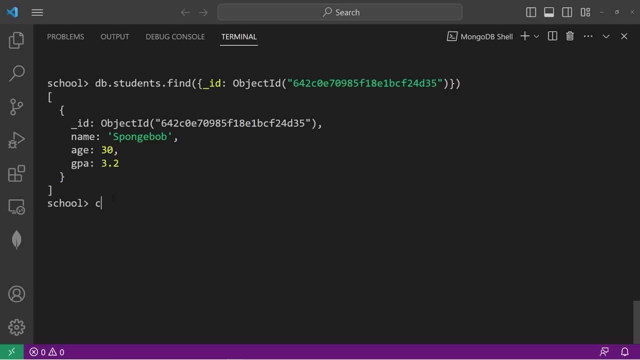 You can use the unset operator to remove a field. Now let's talk about update many. Using the update many method, we can update many documents at once. dbstudentsupdatemany- Let's see- has the same parameters as update1.. If I would like to select every document, I will use an. 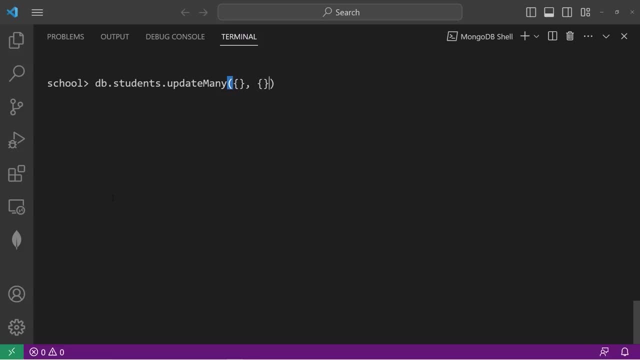 empty set of curly braces. What are the changes we would like to make? Let's use the set operator. Let's set everybody's full time field to be false. If they don't have this field, one will be created for them. All right, let's find every student That was acknowledged. 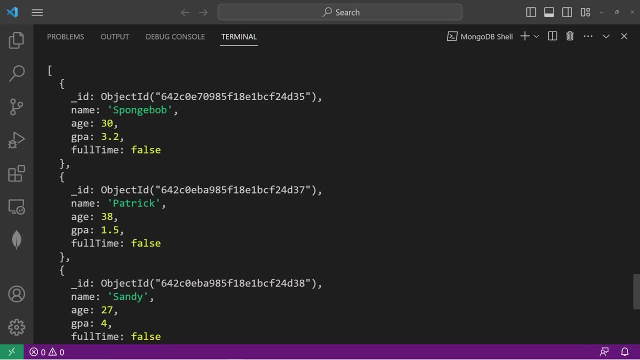 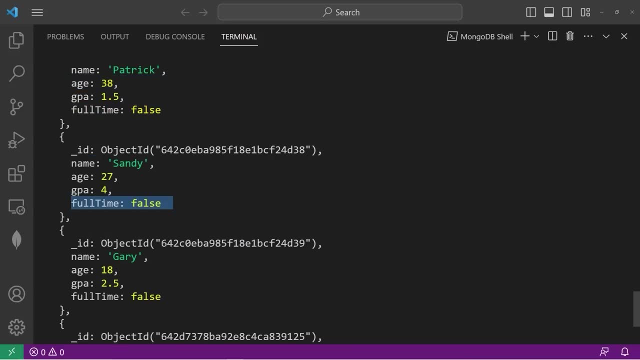 dbstudentsfind everybody. Everybody should have a full time field that is set to false. Full time is false Here as well. Yeah, and that applies to everybody. All right, Let's unset the full time field for Gary and Sandy. dbstudentsupdate1.. Let's select name. 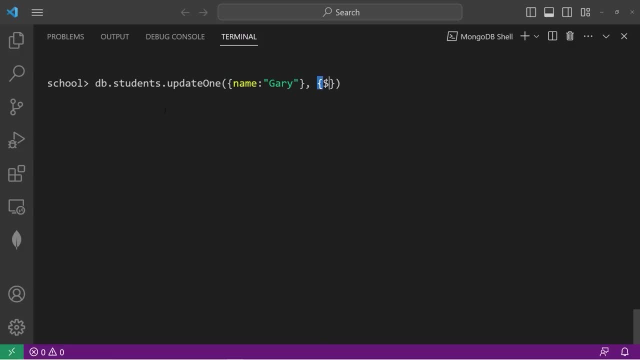 Gary, We will use the unset operator and add the changes to be made Full time. We will remove it by placing an empty string. I am going to copy this line. We will reuse it later. That was acknowledged. Then let's remove full time for Sandy. That was acknowledged as well. Let's double check dbstudentsfind. 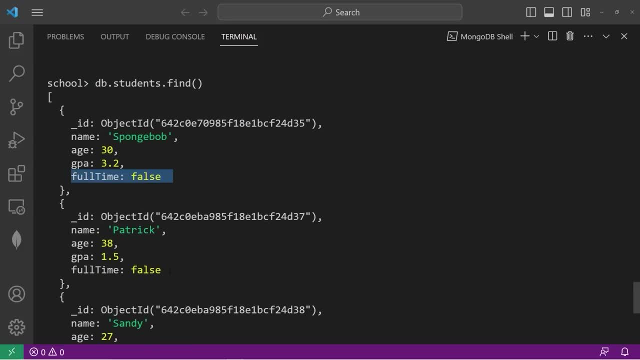 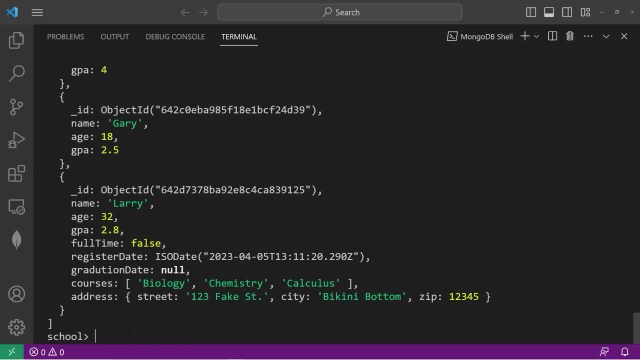 find So. SpongeBob and Patrick both have this full time field, Sandy and Gary don't. They were unset With the update. many method we can check to see if a field exists or doesn't exist within the selection criteria. If any student doesn't have a full time field, let's update it: dbstudentsupdate. 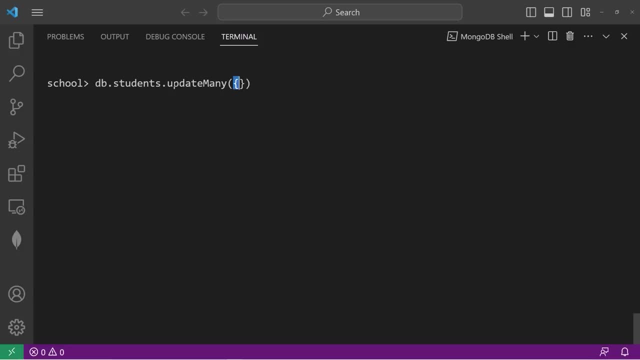 many. What is the selection criteria? Let's say the selection criteria is full time field. Does it not exist? We will use the exists operator, Exists preceded with the dollar sign, Then add false: Does this full time field not exist? That's the selection criteria. If a document doesn't have 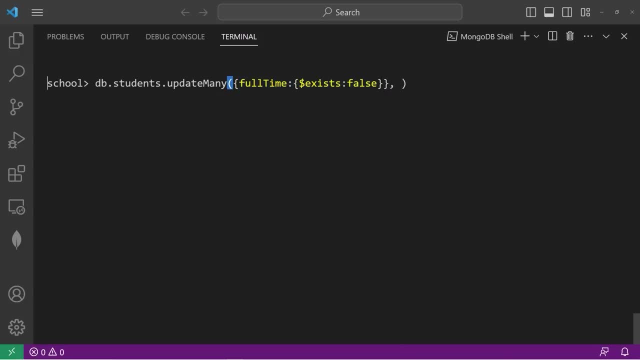 the full time field, we'll give them one. So the second argument will be the changes to be made. We will use the set operator colon: another set of curly braces. Anybody that doesn't have the full time field. let's set that to be true Full. 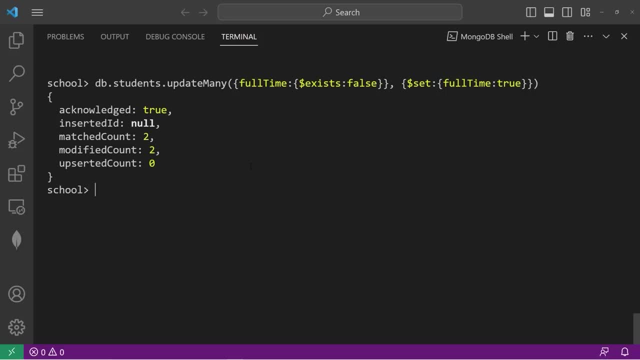 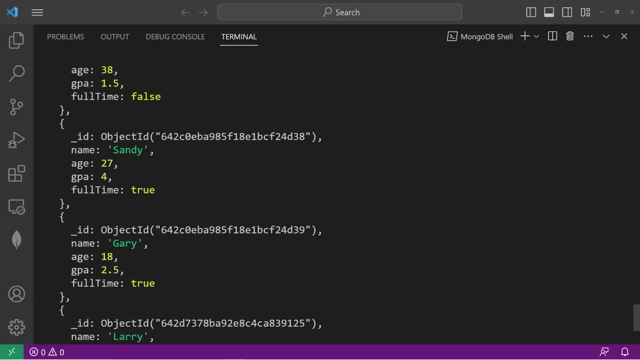 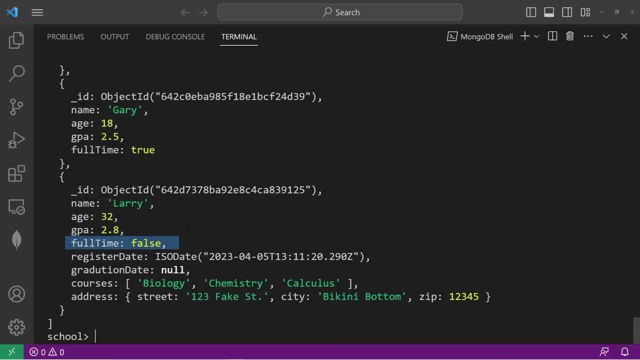 time. true Press enter. That was acknowledged. Let's take a look at our students: dbstudentsfind All right. So Sandy and Gary are both full time students now. SpongeBob, Patrick and Larry are not full time students. They're part time students. That's how to update documents in the MongoDB. 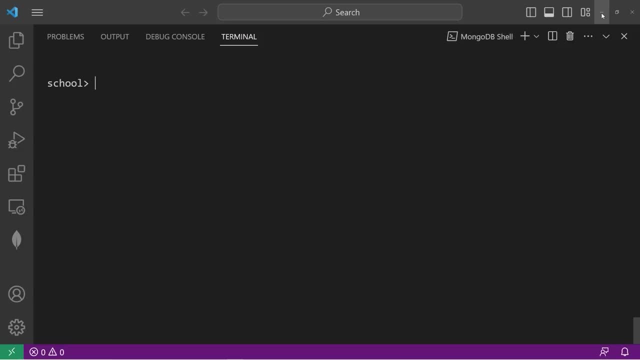 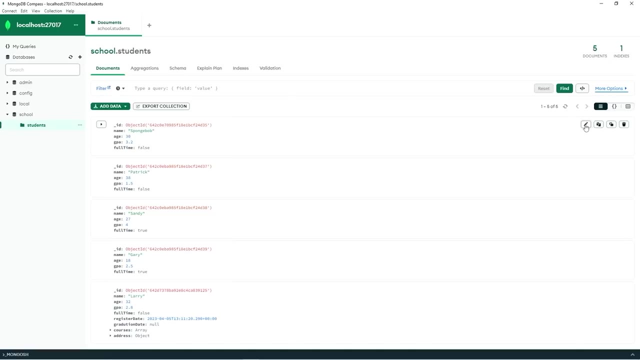 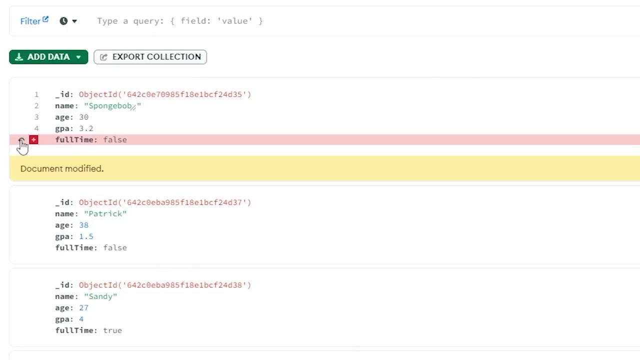 shell. You can use update one or update many. Let's do the same thing with Compass. Hello again everybody. In Compass, to update a field of a document you can press the pencil icon to edit the document. To remove a field next to the field name you can press the trash can icon to remove. 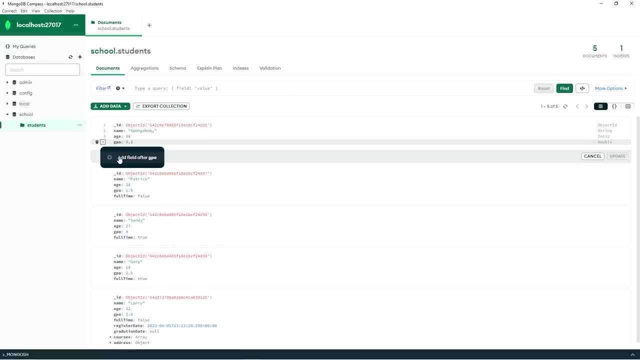 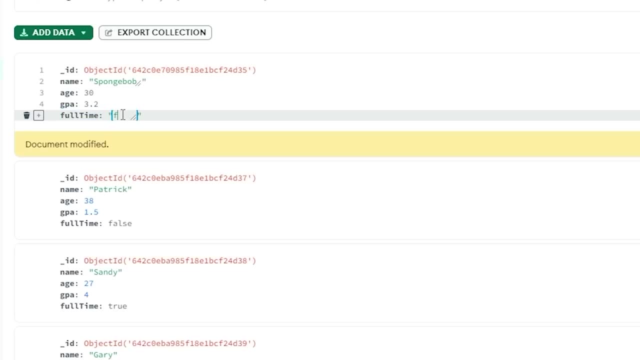 a field To change a field. you can add a new field by pressing the plus button to add a field. Let's add a full time field For the value. I will set that to be false for SpongeBob, Then you can change. 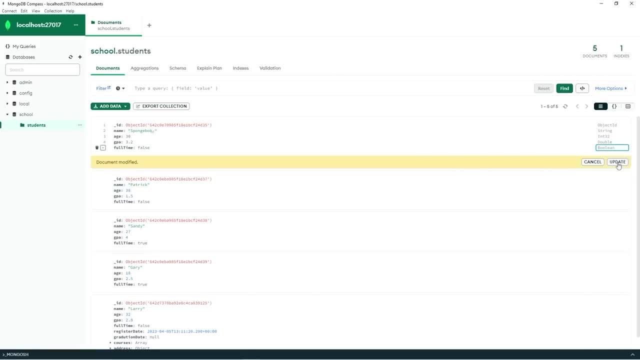 the data type here. We'll change that to be a Boolean. Then update. To change a pre-existing field again, go to the pencil icon, Select your field. Then you can change one of the values. But I'll keep this as false. 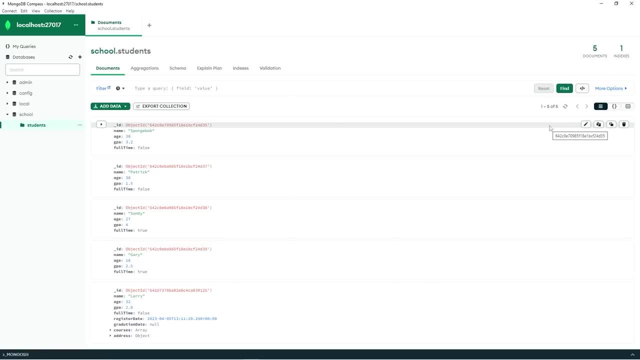 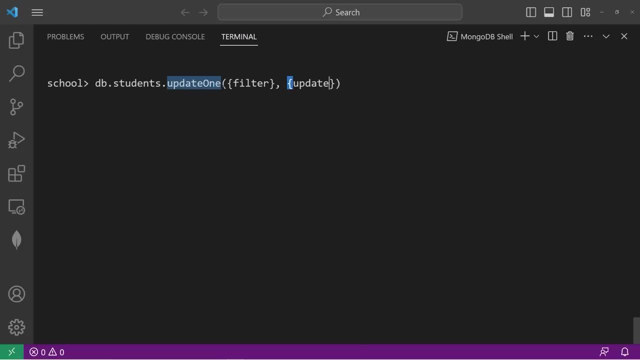 That is how to update documents in Compass. It's fairly easy and straightforward, Alright, everybody. so that is how to update documents in MongoDB. You can use the updateOne method or updateMany. You pass in a filter for the selection criteria, then the modifications within the update parameter. 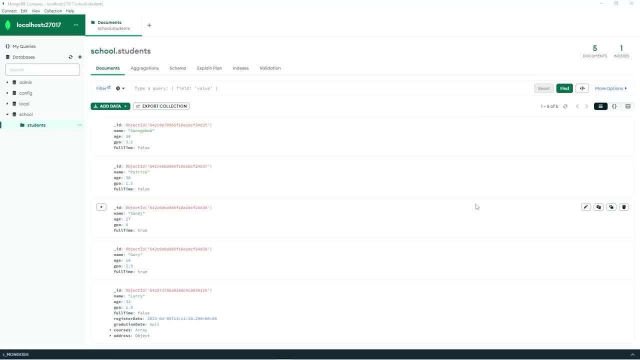 And that is how to update documents in MongoDB. Hello again, friends, it's me again. Today, I will be explaining how we can delete documents in MongoDB. Before we do begin this lesson, I recommend exporting your collection. We'll be deleting documents. 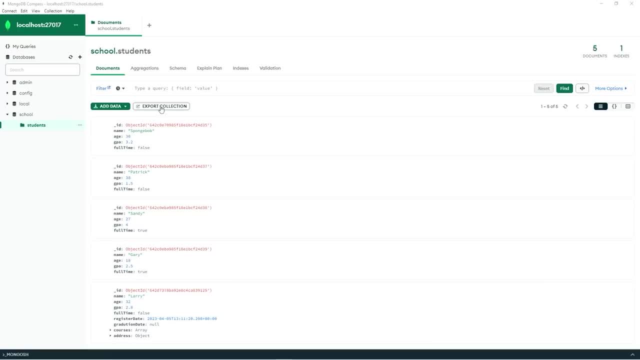 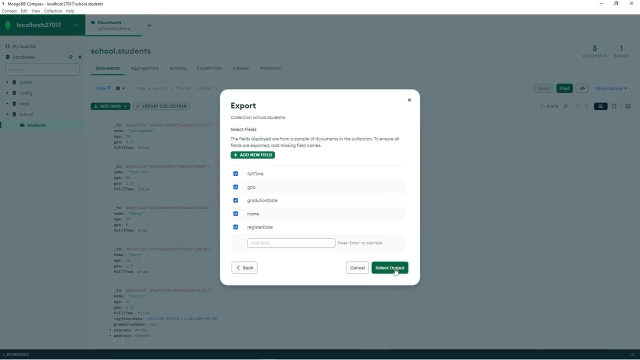 Adding them back in is kind of a pain in the ass, unless we're importing them. So let's export our collection. Export query with filters. that's fine Select output. You can export as a JSON file or as a CSV file. Let's export our collection as a JSON file. 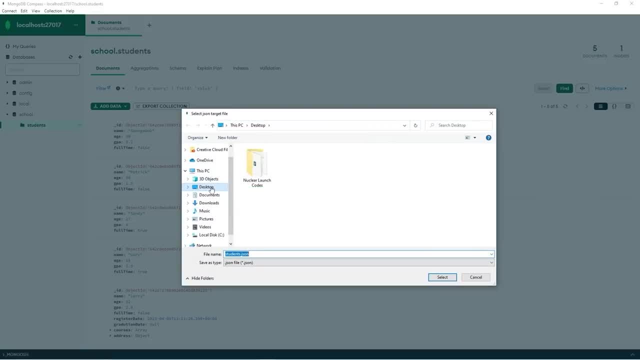 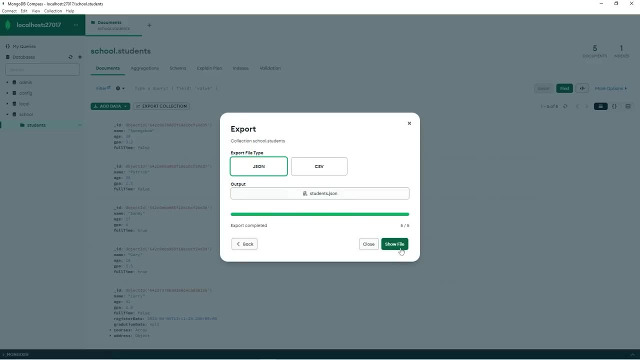 You can also select a destination. I'll place this file on my desktop just for convenience And export. We'll be importing this JSON file at the end of this lesson And close Within Compass. to delete a document, all you do is press the trashcan icon. 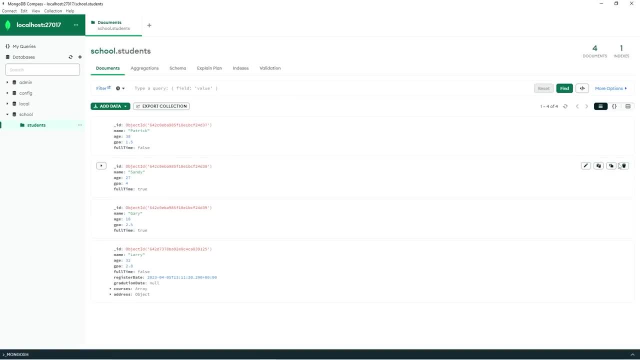 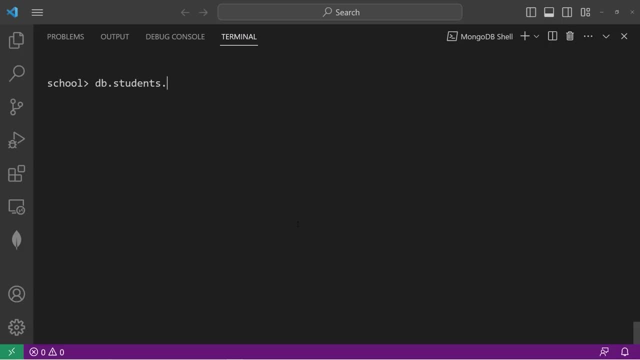 Then delete. It's really easy in Compass In the shell. it's a little different In the shell to delete a document type dbstudents. Then there's deleteOne or deleteMany. We'll begin with deleteOne. We have one person. 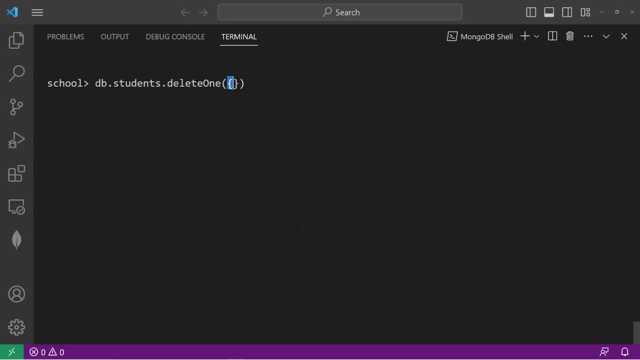 We have a filter parameter, A filter parameter. It's very similar to the find method. We list some criteria to search for. Let's delete anybody with the name of Larry. That was acknowledged. The deleted count is 1.. Let's find our students: dbstudentsfind. 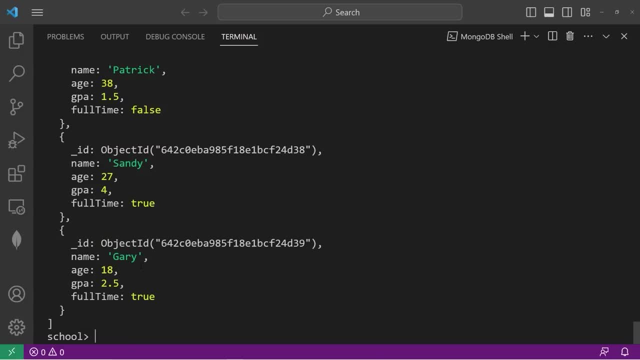 And Larry is no longer at the bottom. We have Patrick, Sandy and Gary remaining. We can use deleteMany to delete more than one document. dbstudentsdeleteMany Pass in our criteria. Anybody that has a full-time field set to false will delete. 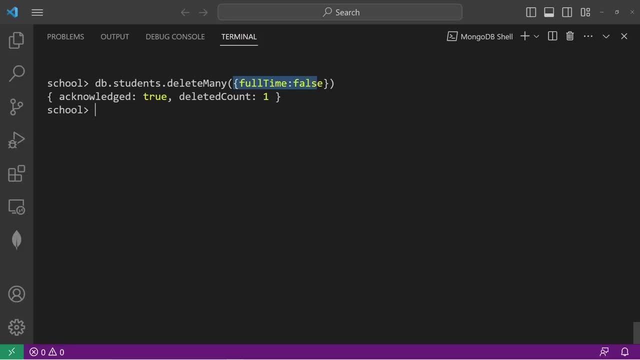 So we have deleted one person that matches this criteria: dbstudentsfind. We have deleted Patrick. We can delete any documents that are missing a field, Or if a field does exist, we can delete that. Let's delete any document that is missing a registration date. 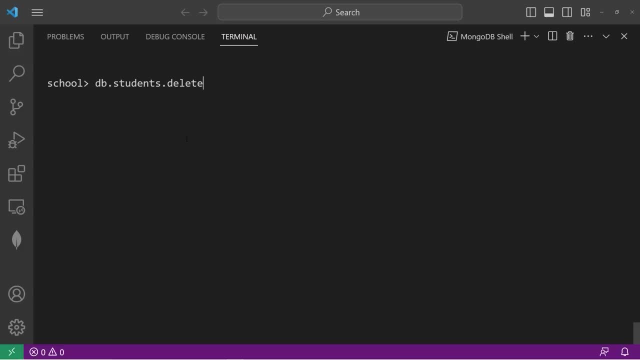 dbstudentsdeleteMany. We are checking if there is a registration date field. Does this field not exist? If it doesn't, then delete that document. We will use the exists operator, colon false. If this field doesn't exist, delete that document. 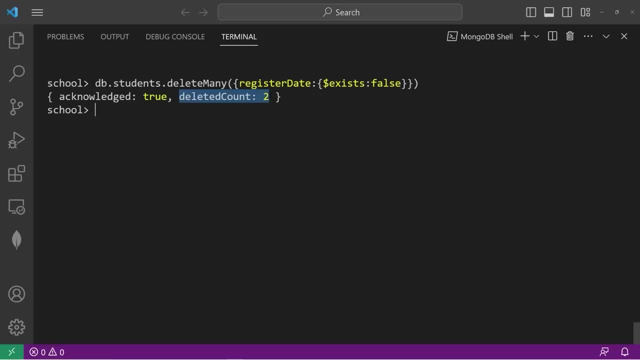 So we have deleted two documents. If we take a look at our students now- dbstudentsfind- We no longer have any students, So that's how to delete one or many documents with the MongoDB shell. Now, if we head back to Compass, 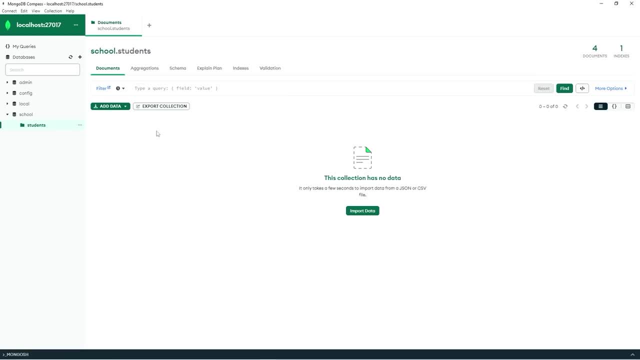 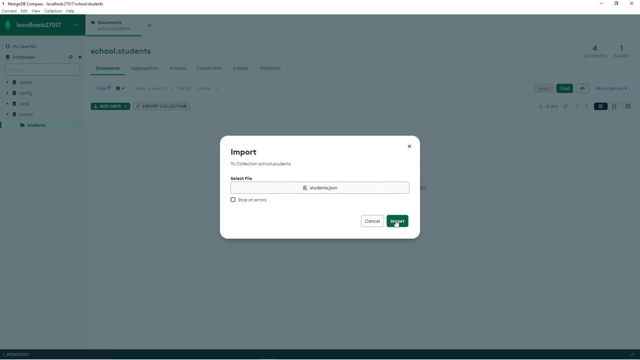 Then refresh. we have no more students. Let's import our collection that we exported, because we do need some data for this series. Add data, Import JSON or CSV file. We are looking for our students JSON file, Select And import And we're done. 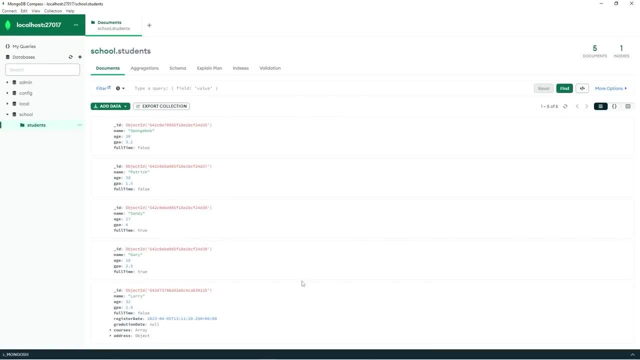 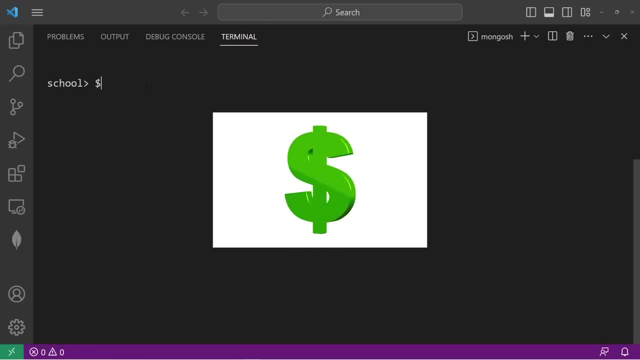 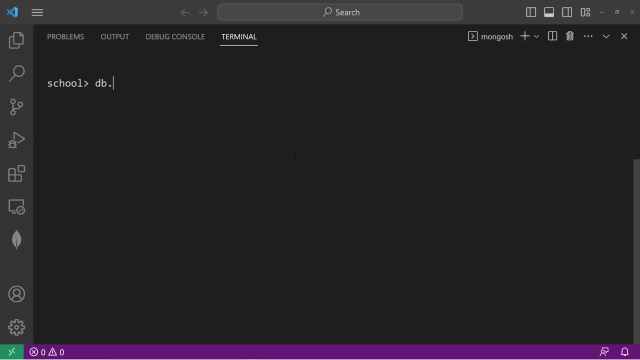 So that is how to delete documents in MongoDB. Hey everyone, today I need to explain comparison operators. Operators are denoted with the dollar sign. Comparison operators return data based on value comparisons. In previous examples we would type dbstudentsfind, Then list some criteria. 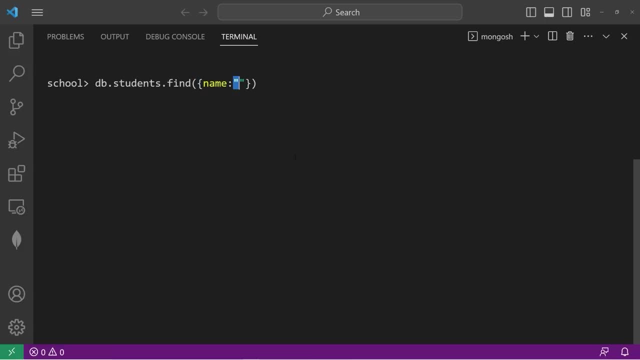 Like, if we're looking for Spongebob, we would say: name Spongebob. Now what if you would like to find everybody but Spongebob? Well, you can use the not equals comparison operator. We would enclose it within a document body. Pre-seed our value with the not equal comparison operator. 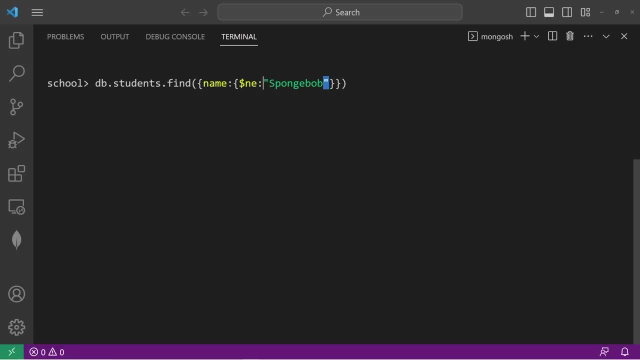 Dollar sign and E colon. Find every name that's not Spongebob. That gives us four. That gives us four records: Patrick, Sandy, Gary, Larry. Spongebob isn't within here. That is the not equals comparison operator. Return every document that has a name not equal to Spongebob. 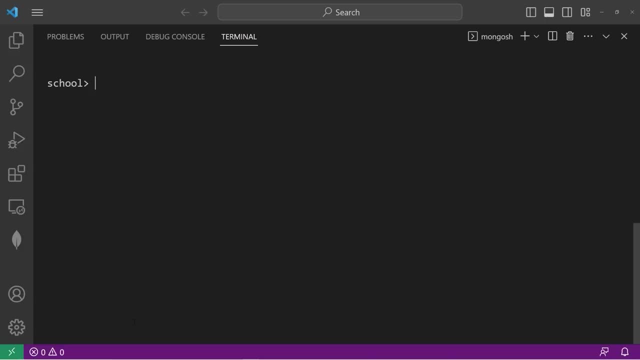 Let's go over a few more. Let's cover less than and less than equals too. dbstudentsfind- Find everybody that has an age That is less than So. dollar sign LT for less than 20.. That gives us one document, Gary, who's 18.. 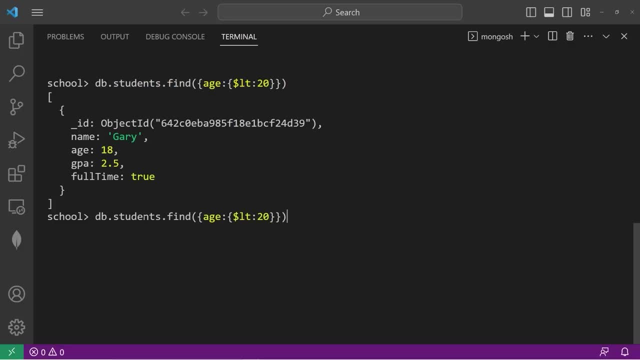 Or we could use less than equal to Change LT to LTE. That means our 20 is inclusive. Maybe let's change this to 27.. Return every document where the age field is less than or equal to 27.. That would give us two results. 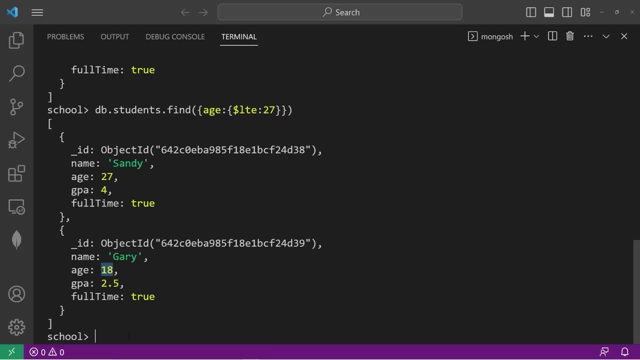 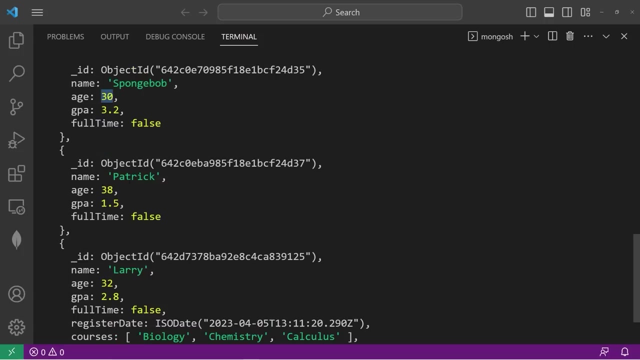 Sandy, who's 27 exactly, And Gary, who's 18.. Let's do greater than Return every document where age is greater than 27.. That gives us three documents: Spongebob, who's 30.. Patrick, who's 38.. 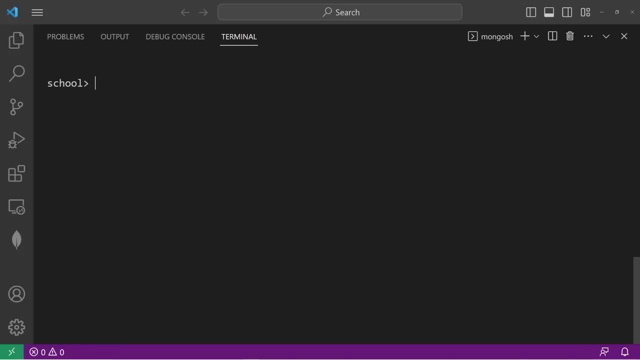 Larry, who's 32.. Let's do greater than equals. That would be GTE: Find everybody that's greater than or equal to 27.. That gives us four records: Spongebob: Patrick, Sandy, who's 27 exactly. 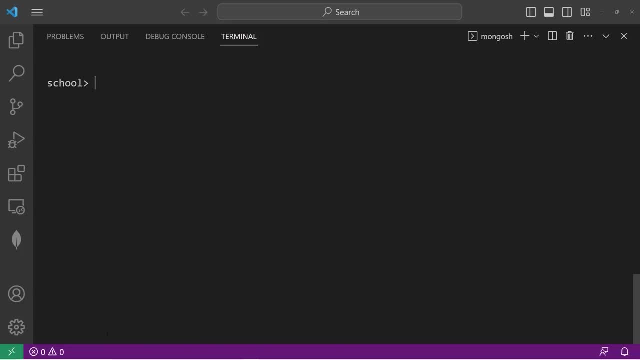 And Larry. So that's less than less, than equals to greater than and greater than equals to. You can use more than one comparison operator to find values within a certain range. Let's find every student whose GPA is between 3 and 4.. 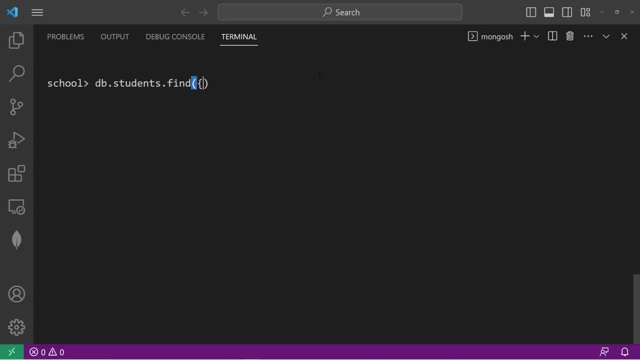 dbstudentsfind. We are searching for GPA. Let's use the greater than equals to comparison operator. Return every GPA that's greater than 3. Comma And less than or equal to 4.. So these would be the students that have a good GPA. 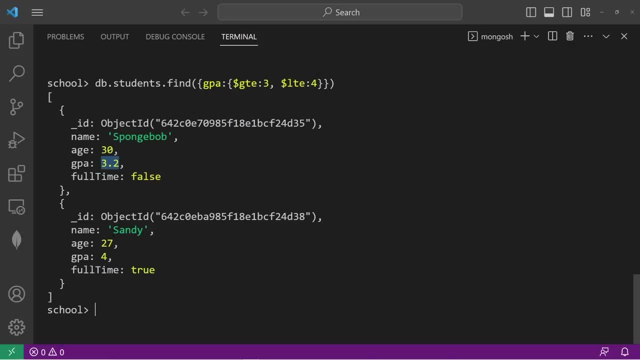 Spongebob and Sandy. Spongebob has a GPA of 3.2.. Sandy's is 4.0.. You can use more than one comparison operator To give you a range. Now, another good operator is the in operator. With the in operator, we can return all records that have one of these matching values. 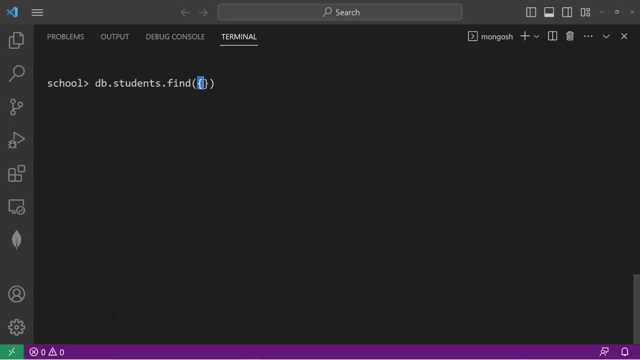 So dbstudentsfind, Let's find any student whose name is within this array. We will pass in a document body, Use the in operator, Then list an array, An array of values. Let's find anybody whose name is either Spongebob, Patrick or Sandy. 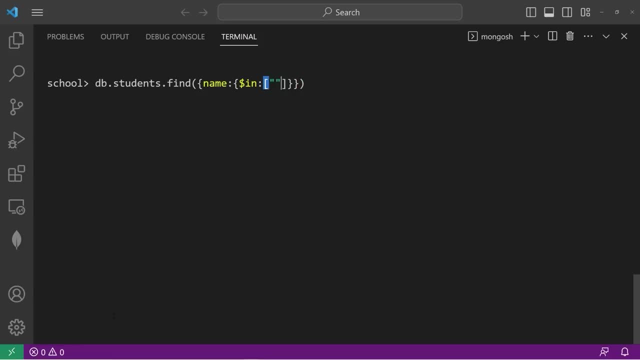 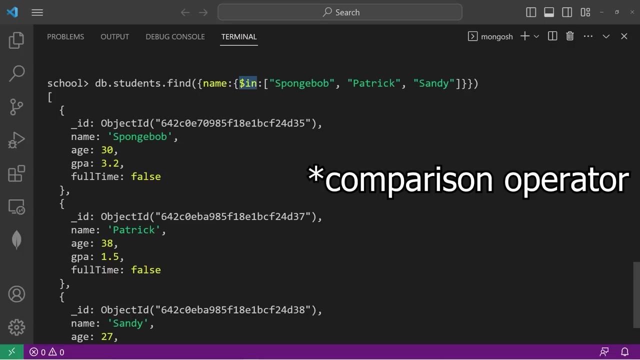 So within an array we will list our values. Return anybody whose name is Spongebob Patrick or Sandy There. Spongebob Patrick, Sandy. With the in logical operator, you will return all documents where one of the values in this array. 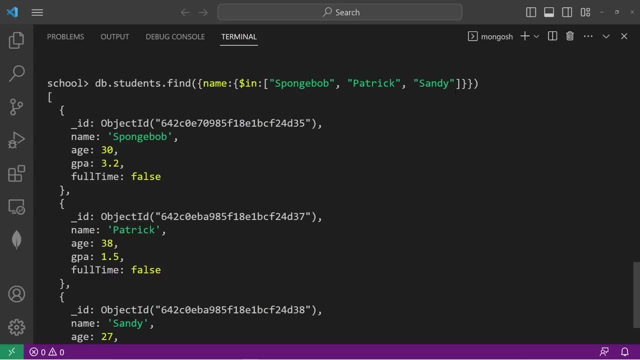 In this array Is found within this field. You can also use not, in, Which is nin. So let's copy this line. Clear our screen, Paste it, Change in to nin: Not in Return all documents where name doesn't have one of these values. 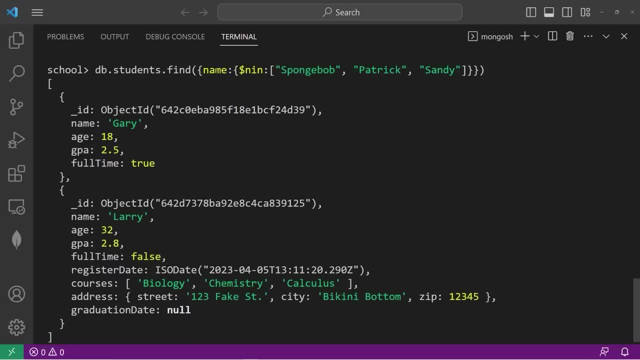 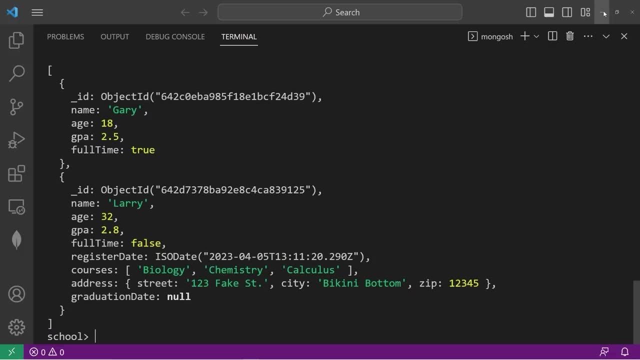 That would give us Gary and Larry. We are given everybody's name. That's not Spongebob, Patrick or Sandy. Let's switch to Compass and I'll show you how we can do the same thing Within Compass. you would write your filter within this text box. 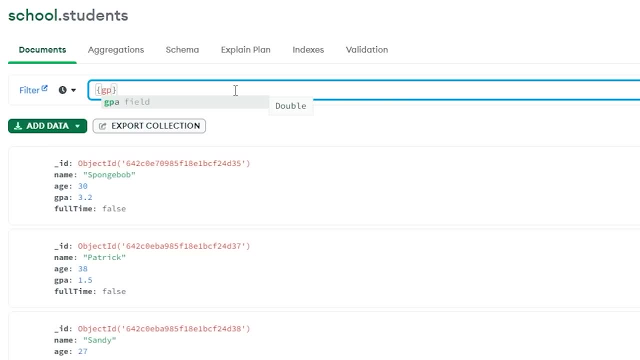 Return everybody who has a GPA field That is greater than or equal to three- GTE Three. That gives us Spongebob and Sandy. Give us everybody whose, let's say, age Is less than 27.. That gives us Gary. 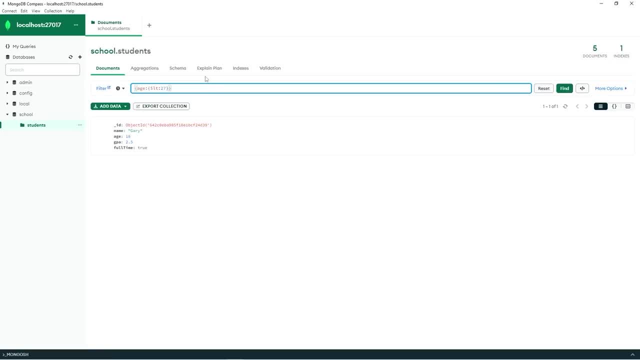 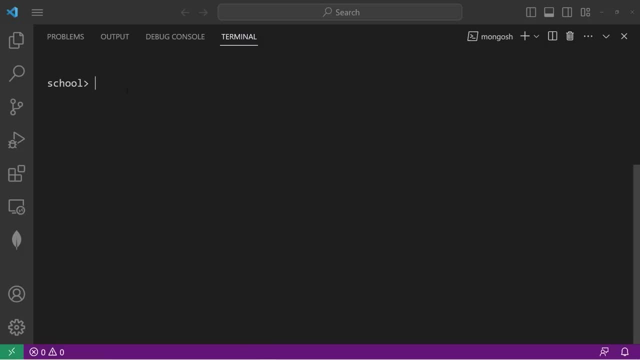 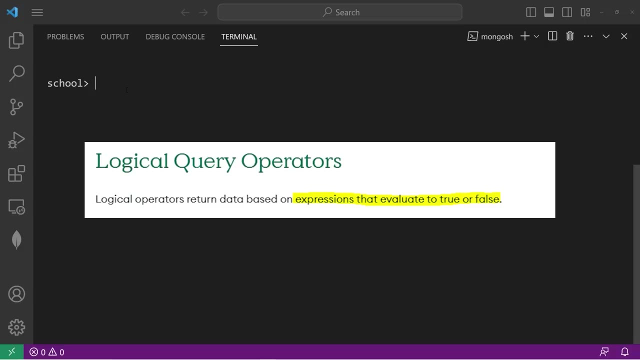 Alright, everybody. so, in conclusion, comparison operators return data based on value comparisons, And those are comparison operators in MongoDB. Hey, everybody, today I need to explain logical operators. Logical operators return data based on expressions that evaluate to be true or false. There's four. 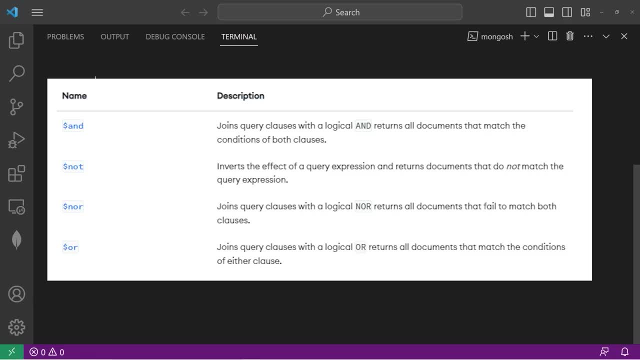 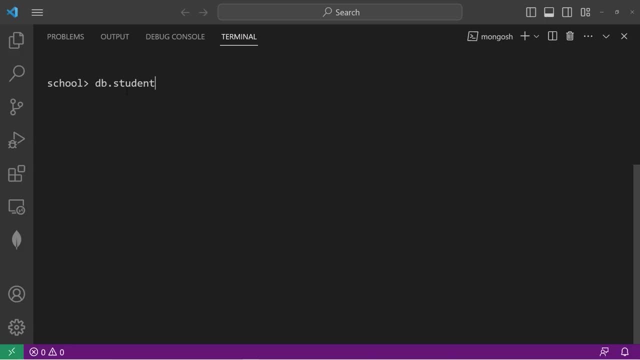 And or nor and not. Let's begin with and Using the and logical operator, we can check to see if two expressions are true. Let's begin with: dbstudents. That's the name of the collection. We'll use the find method. 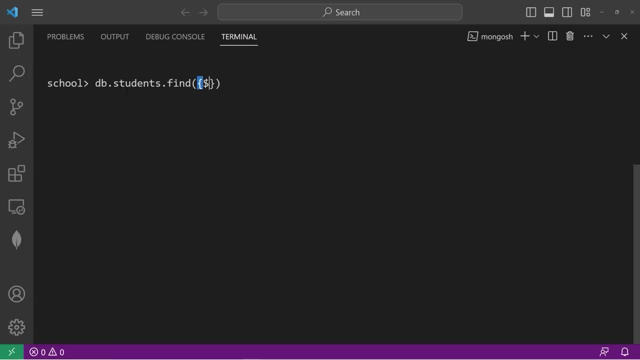 Pass in a document. object: We will use the and logical operator. It's preceded with a dollar sign. It's an operator, Then a colon. Whatever expressions you would like to check. you will place within an array List as many expressions as you would like. 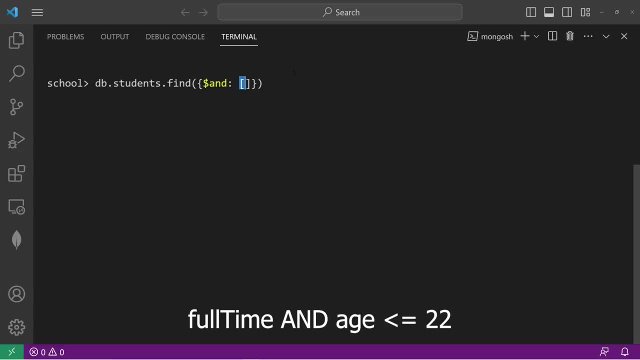 Let's return any document where the student is a full-time student And they're 22 years or younger. Usually most students, when they start college, they're between the ages of 18 and 22. So let's find all those students. 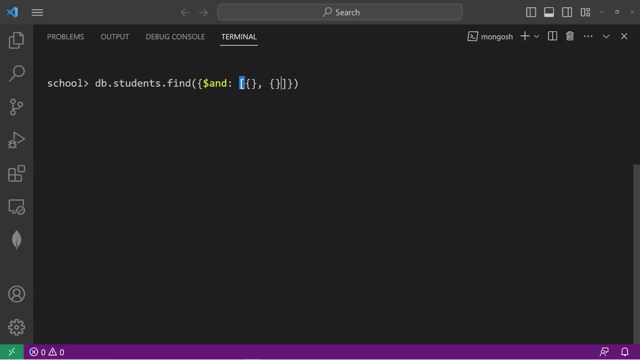 We'll have two conditions. We need two document bodies. Our first condition is full-time. true, Give me any student that's a full-time student. And our other condition is: give me any student that's age is less than or equal to 22.. 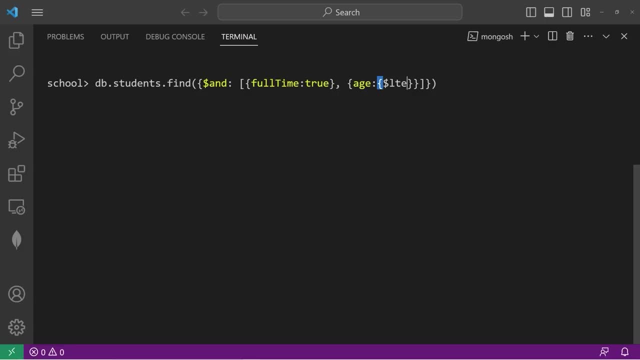 We'll use the less than equals comparison operator, colon 22.. And that's it. We have one student, Gary. He's 22 and under and a full-time student. So with the and logical operator you can have more than one condition. 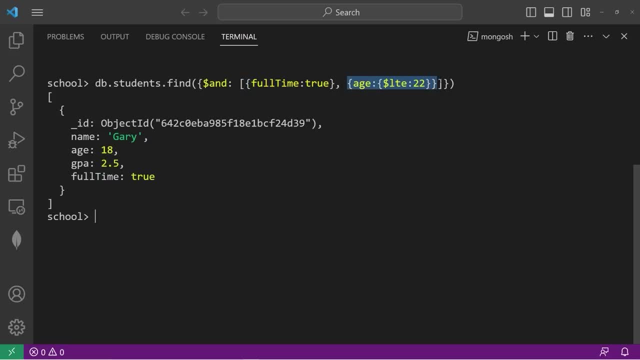 This condition needs to be true. This condition needs to be true And that condition needs to be true. We were given the result of Gary. He's the only student that passes these two filters. They both evaluated to be true. Let's copy this method. We'll reuse it. 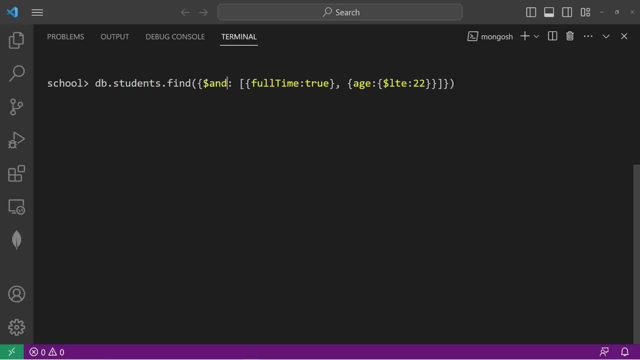 Let's discuss or Change and to or With the or logical operator. at least one of these conditions need to be true. Give me anybody that's a full-time student Or anybody that's 22 or younger. That will give me two documents. 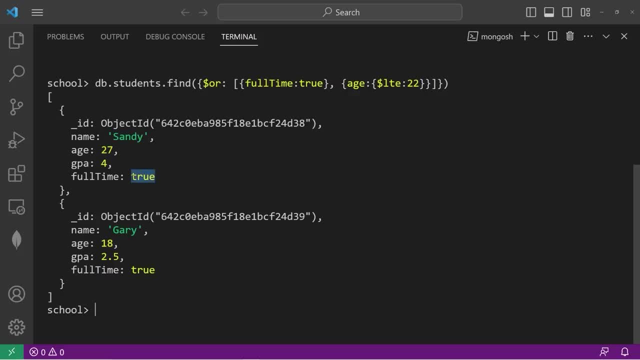 Sandy. she's older than 22,, but she's a full-time student. Gary is 22 and under and a full-time student. So with the or logical operator, at least one condition needs to be true. So again, let's copy this method. 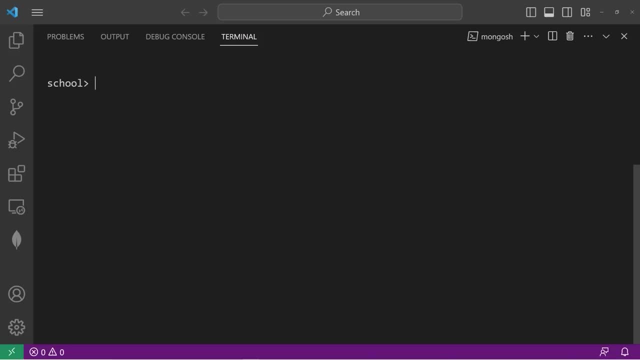 We'll reuse it. Then we will talk about nor So with the nor logical operator N-O-R. we will return any document where these conditions are false. This needs to be false As well as this needs to be false. It's kind of like and, but instead of both conditions being true, it's the opposite. 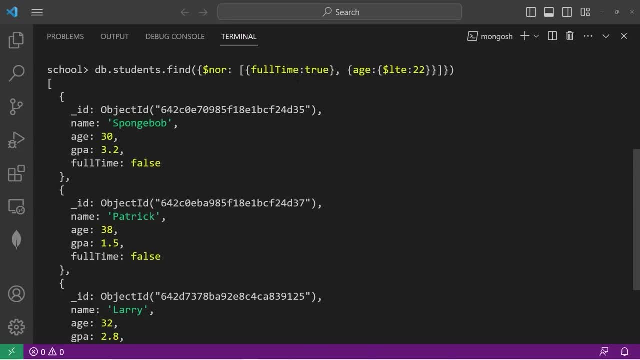 They both need to be false, So that would give me three results. SpongeBob, he's above 22.. He's a part-time student. Patrick is 38.. He's a part-time student. Larry, he's 32.. He's a part-time student. 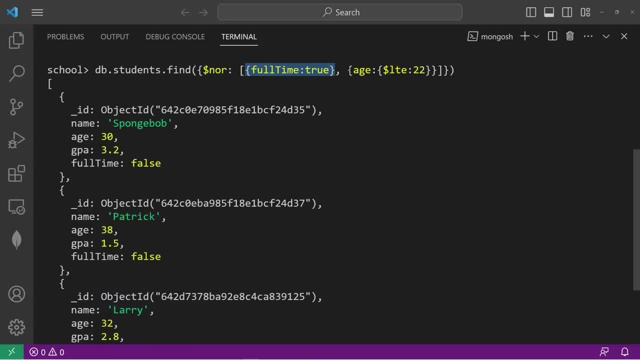 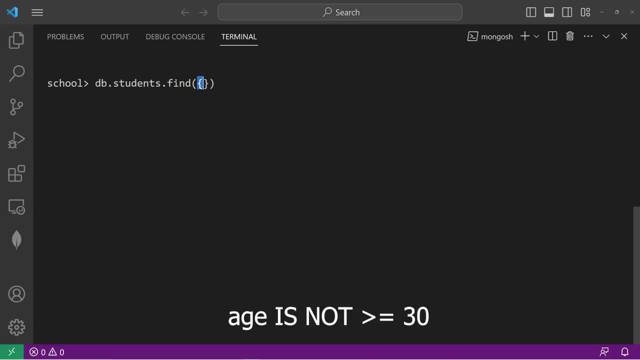 With the nor logical operator. we need both of these conditions to be false. That gave us these three documents for SpongeBob, Patrick and Larry. Lastly, we have not- Suppose I have this query- dbstudentsfind- Find any student that is not above 30.. 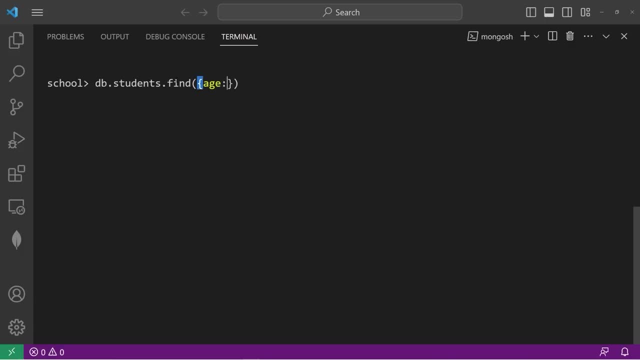 I could write something like this: Age colon: we'll use the less than comparison operator, colon 30. Find any student under 30. Normally this would give me Sandy and Gary. You know this does work, but what if somebody doesn't have some information for their age? 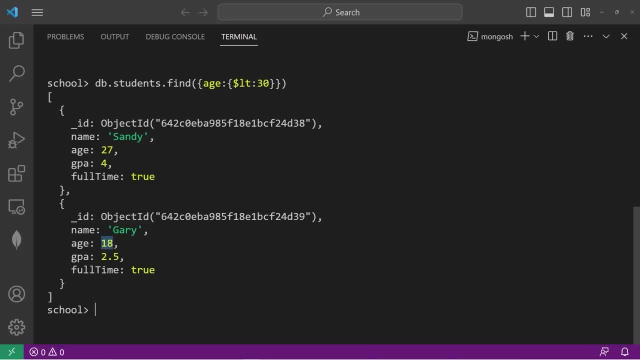 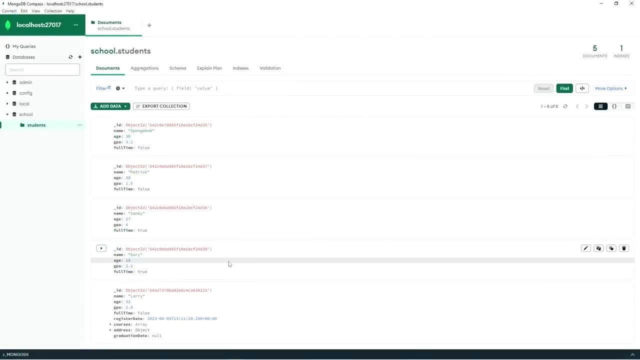 Like, let's change Gary's age to null, Because in SpongeBob lore Gary is a pet snail. His age is in cat years. Just to make this easy in Compass, I'm going to edit Gary's age to be null. 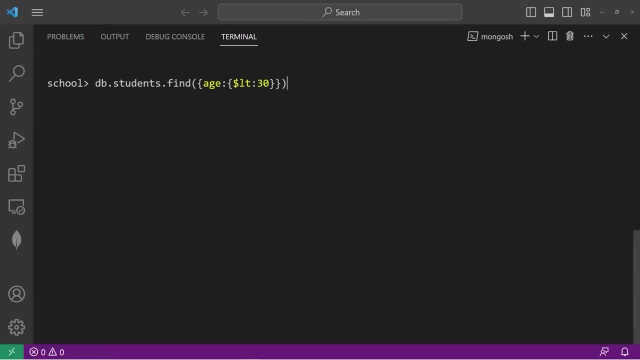 Let's write that query again: Give me any student whose age is less than 30. Well, that only gives me Sandy Gary's age is null. So another way in which we could return all students that are not 30 or above. 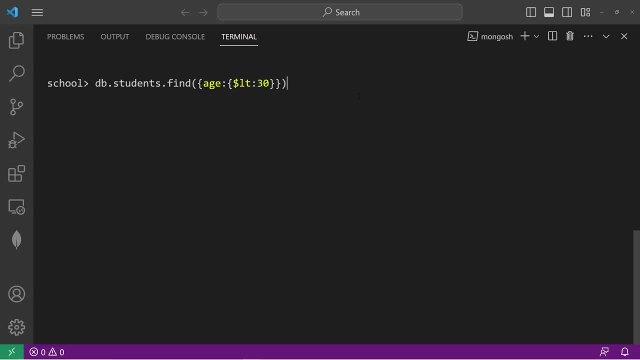 we can use the not logical operator. The not logical operator reverses what you're looking for, So let's enclose this document body within another document body. Then we will use the dollar sign, not logical operator, But we will change the comparison operator to be greater than either. 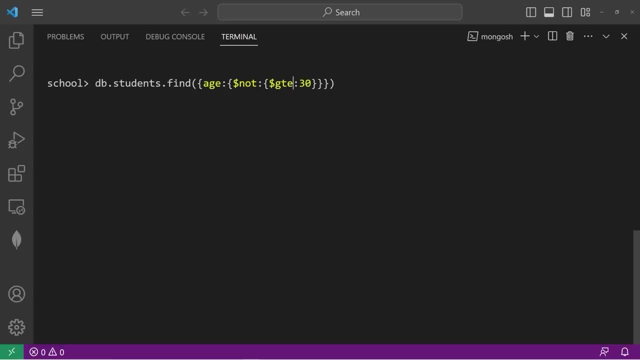 Greater than equals. Give me any student that is not greater than or equal to 30. So that should give me both Sandy and Gary, even though Gary's age is null. In many circumstances you could use less than, But a benefit of the not logical operator is that it would give you null values. 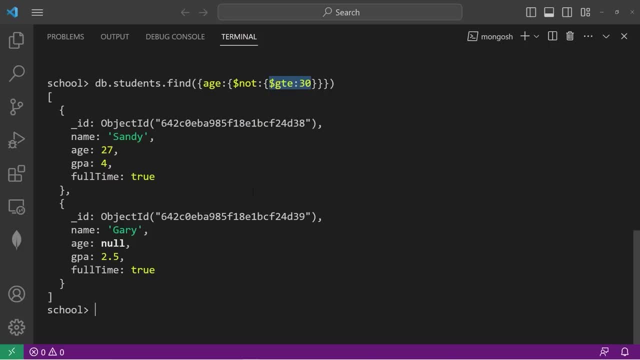 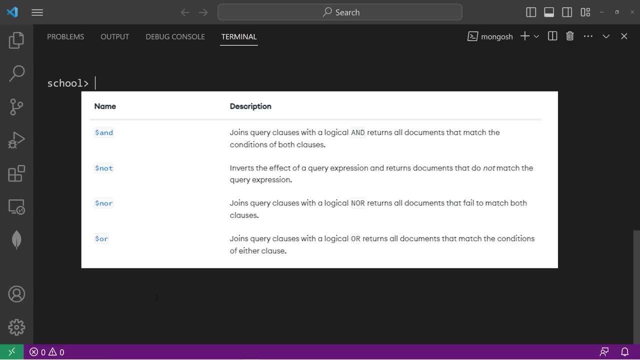 Return any document that doesn't fit this condition, Basically speaking, not just does the opposite. Alright, everybody. so those are logical operators. They return data based on expressions that evaluate to be true or false. And those are logical operators in MongoDB. Hey, everybody, today we are moving on to indexes. 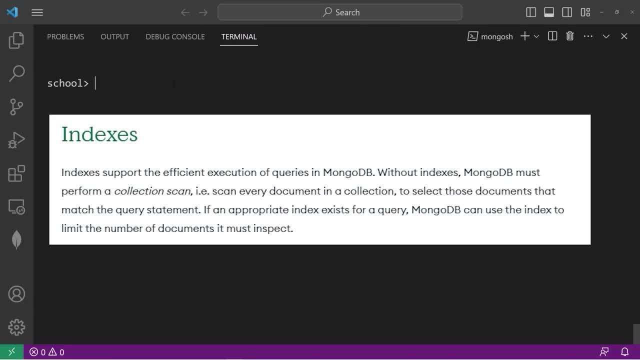 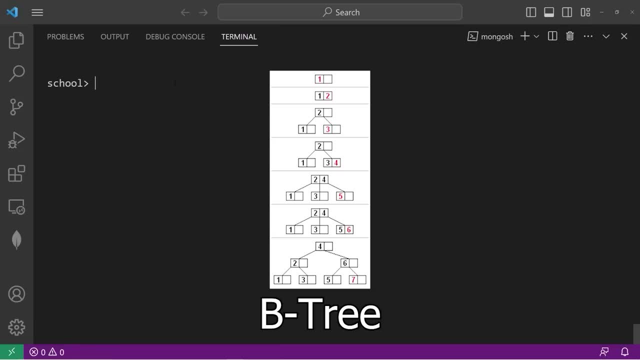 An index allows for the quick lookup of a field. However, it takes up more memory and slows insert, update and remove operations. Use them wisely, Utilizing an index if you're familiar with data structures and algorithms. we're storing our data as a B-tree. 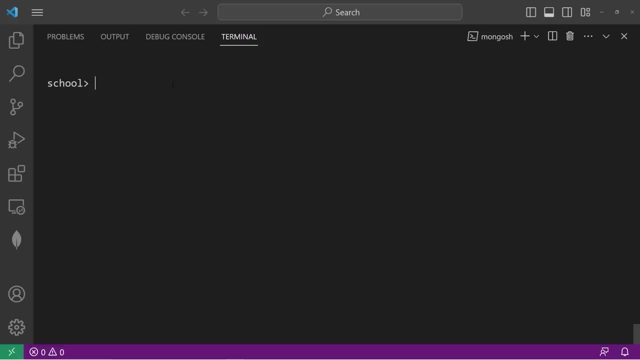 If there's a field you search for but you don't do many updates, I would recommend an index. Here's an example. Let's find any students named Larry: dbstudentsfind. Find anybody named Larry. I'm going to make one adjustment though. 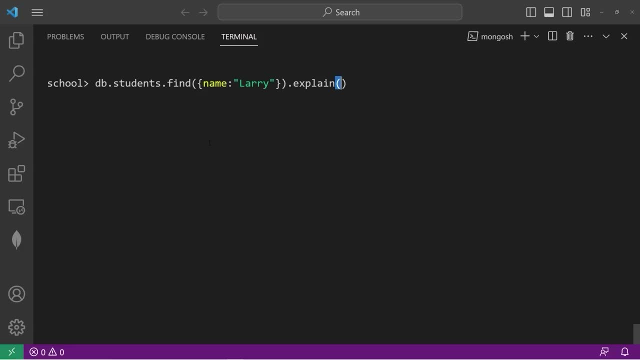 Let's method chain the explain method And pass in this string ExecutionStats. That will give me the execution stats of this query. I have five documents within my collection. We have examined five documents to find Larry. We're performing a linear search through our collection. 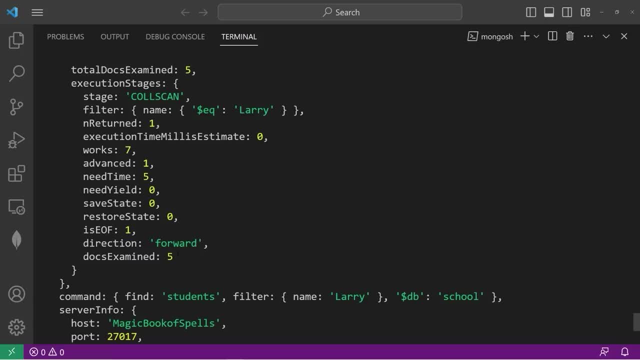 We're examining each document one by one. I only have five documents. That wouldn't take too long. Imagine I have thousands or hundreds of thousands of documents. Well, a linear search is going to take a really long time. We can speed up the lookup process by applying an index. 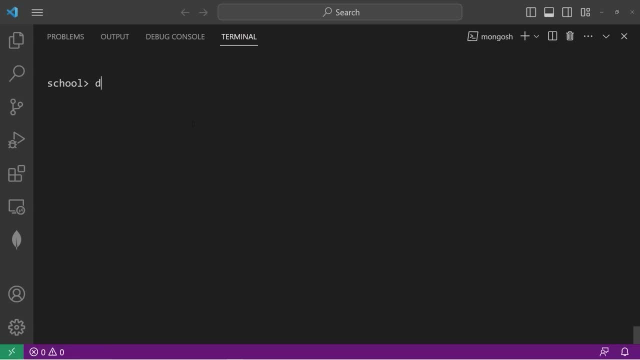 To apply an index to a field. you would type something like this: dbtheNameOfTheCollectioncreateIndex. Now, what field would you like to apply an index for? Let's apply an index to our name field. Name colon. You can arrange the data in your index in ascending order by using 1,. 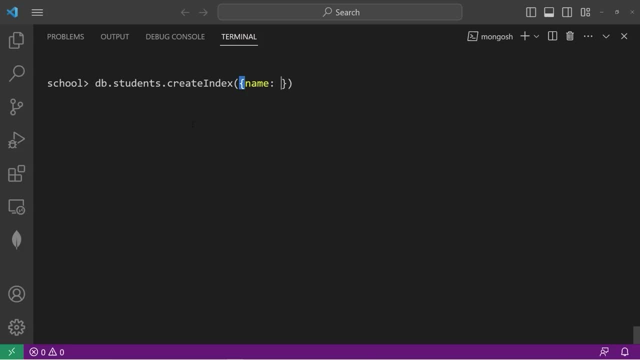 or descending order, with negative 1.. So with a name, 1 would be alphabetical, Starting with A to Z. Let's hit enter. This is the name of our index Name, underscore 1.. Let's perform that query one more time. 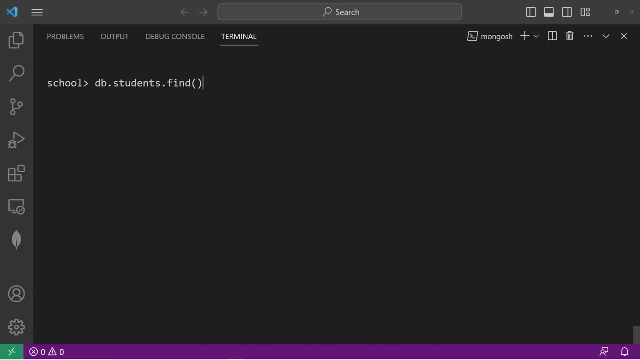 dbstudentsfind. Find anybody named Larry. Name Larry, Then we will method chain the explain method. Pass in the string executionStats. Let's see what the results are. This time we only have one. We only examined one document. Examining one document is a lot less time consuming than examining five documents. 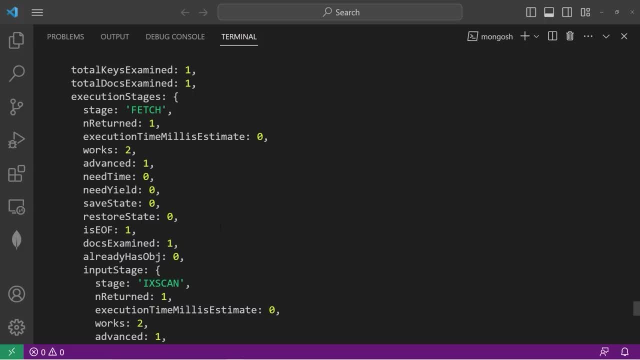 Like I said, I have a small data set. It doesn't appear to make that big of a difference, but if you have hundreds of thousands of documents, it's going to save you a lot of time. To get all your indexes, you can use the getIndexes method. 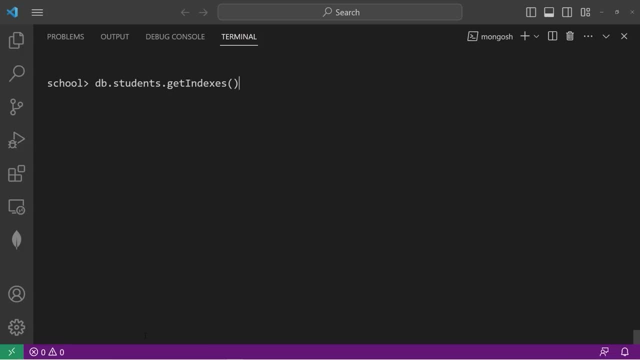 dbstudentsgetIndexes And we have two. There already is an index applied to object ideas. We have that by default And here's the index we created to look up names quickly. We have two indexes. technically, To drop an index you'll need the name. 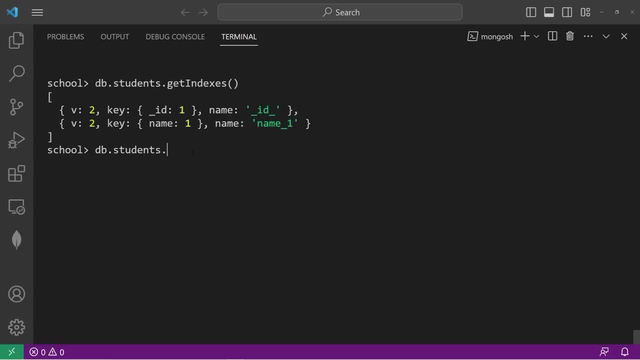 Let's copy that: dbstudentsdropIndex, Place the name of the index within the dropIndex method And our index is dropped. Let's take a look at our indexes again: dbstudentsgetIndexes- And our index is gone. Now, if you would like to create an index in Compass, 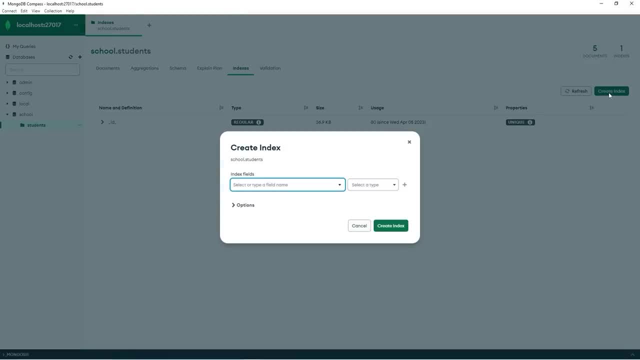 you go to the indexes tab, Create index. Select a type or field name. Let's create an index for name. Select a type. Let's place our name in ascending order. You can select more options, but that's a little advanced for us at this level. 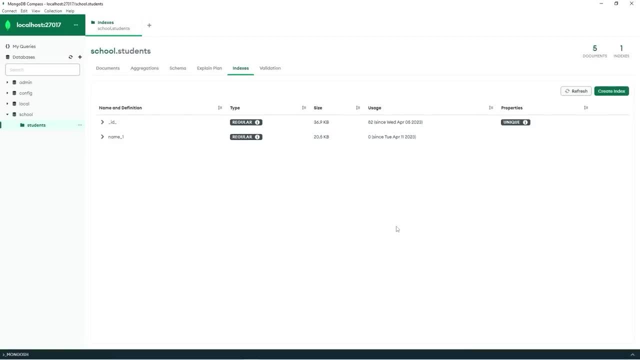 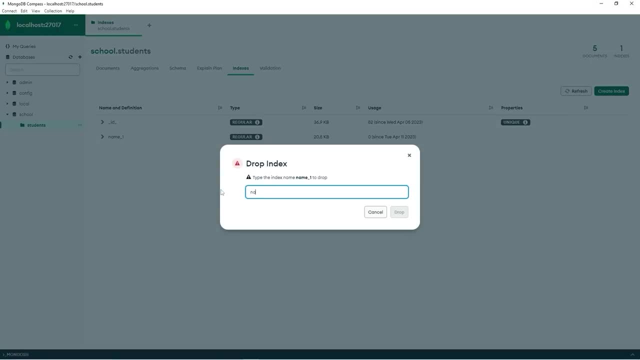 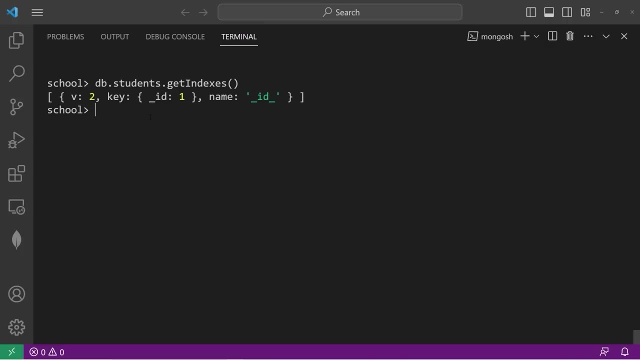 Let's begin with the basics, And that's how to create an index in Compass. Then, to drop the index, you just press this trashcan icon, Type the index name Name, underscore one, And that's how to drop an index. So, in conclusion, applying an index to a field allows for quick lookup of that field. 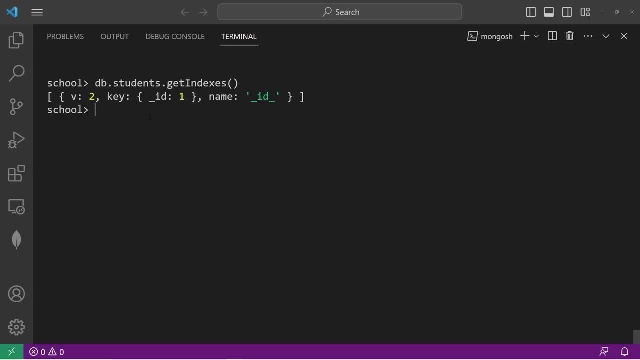 But it takes up more memory And it slows insert, update and remove operations Because you have to update the binary search tree. Use indexes wisely. Personally, I would recommend an index if you're doing a lot of searching but not a lot of updating. 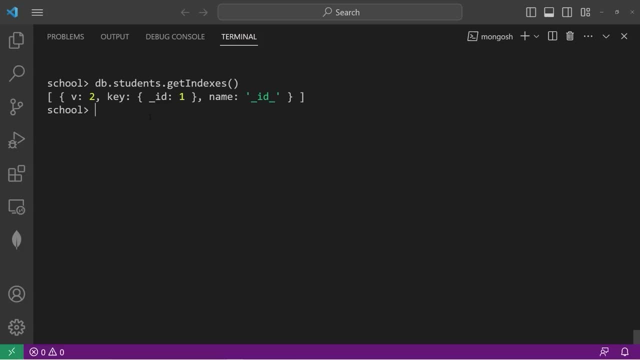 So that's an introduction to indexes in MongoDB. Hey everybody, With the last few minutes remaining of the MongoDB in one hour series, I thought I'd get a little more in depth with collections. As we've learned at the beginning of the series, a collection is a group of documents. 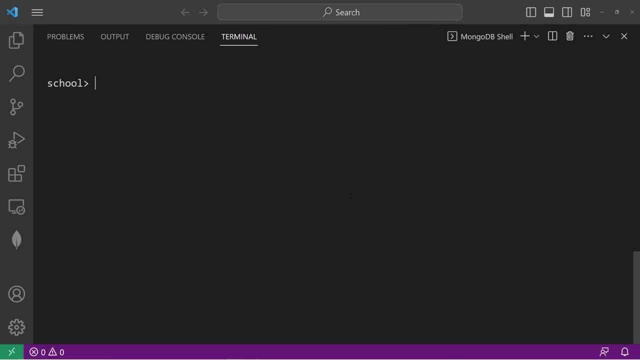 And a database is a group of collections Within your database. to show collections, you can type show collections. Currently we only have one: Students. Let's create another, though. Let's create a collection of teachers. We'll use the dbcreate. 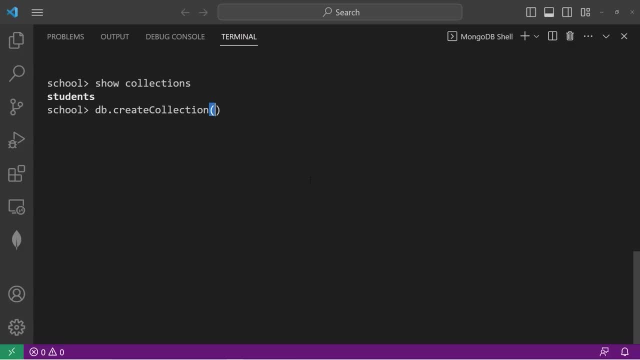 Collection method. Pass in a name for this collection. Let's create a collection of teachers, So this would work. However, there are some additional options that we can pass in as arguments to this method. Let's add the next argument. It's comma separated. 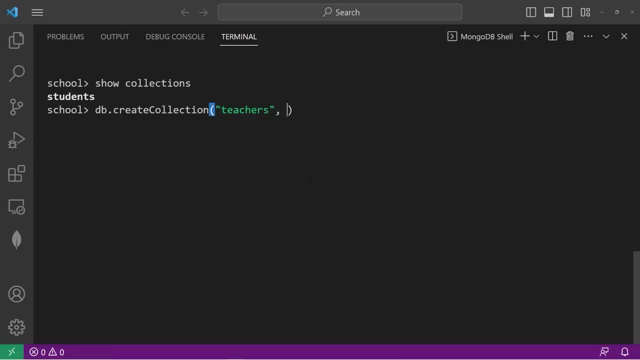 Another argument that we can pass into this method when creating a collection is a max size for this collection. We will set the capped field to be true. That's informing MongoDB. This collection should have a max size. This field is either true or false. 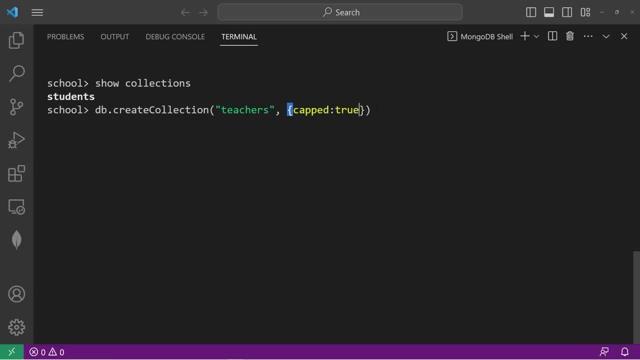 If capped is set to true, you do need a minimum size specified. So size, that's a field. Then set a size in bytes. If you would like a maximum size of 10 megabytes, that would be 10 million, 10 million bytes. 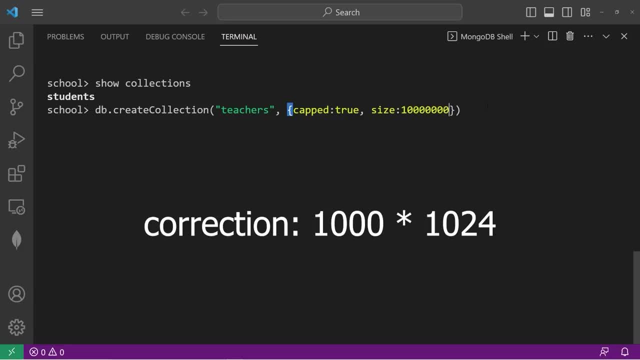 Let me count my zeros. Yeah, that's accurate. And or you can have a maximum number of documents. You will set the max field to be some amount of documents. I don't want any more than 100 teachers. Our collection has a maximum size of 10 megabytes.